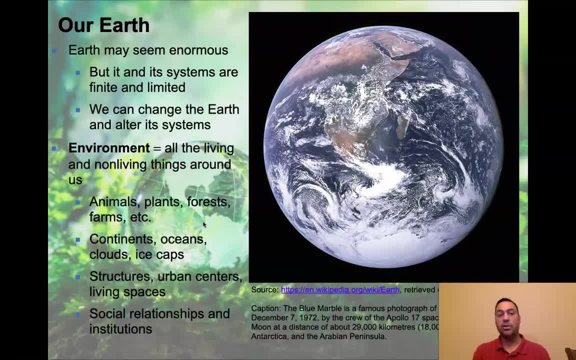 around us. This includes animals, plants, the forests, farms. It can include continents, oceans and clouds, ice caps, In fact. that's what we see here in this picture. This is Antarctica down here, This white down here, of course, being the ice caps. This is Africa, located right here, the island of Madagascar. 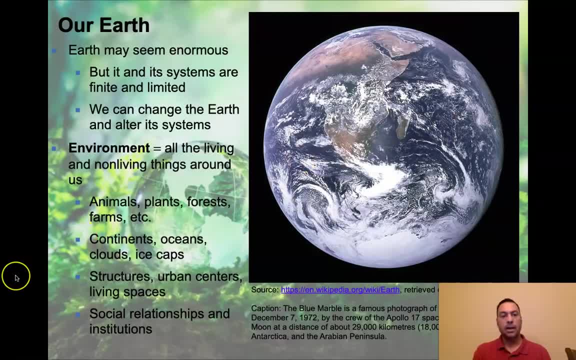 the Indian Ocean here, the Atlantic Ocean over here. So that's all part of the environment. It also includes structures, urban centers and living centers, which include the very building or the outside area where you might be sitting right now watching this video. It also includes 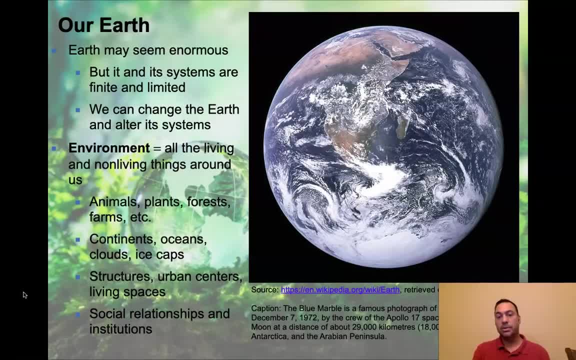 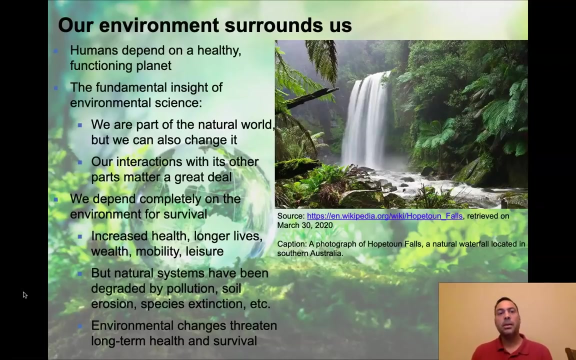 the social relationships and institutions. This includes governmental institutions, corporations and the way that people interact, say through markets, So it all comes together. That's what we mean by the environment. It's everything coming together: the earth, the atmosphere, the biosphere and human behavior interacting with all of those things. Now the 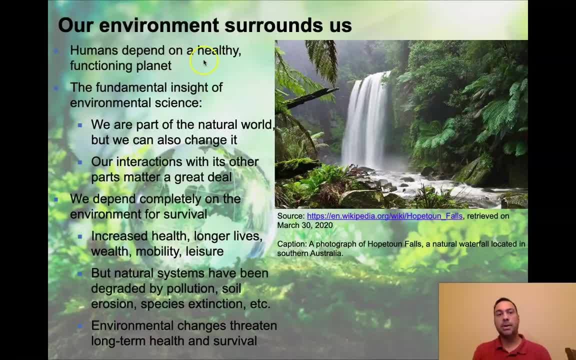 environment. not only does it surround us, but it's important to us because humans depend upon a healthy, functioning planet. Without a healthy functioning planet, we don't get what we call ecosystem services. We'll be talking about this a little bit later on Ecosystem services that keep. 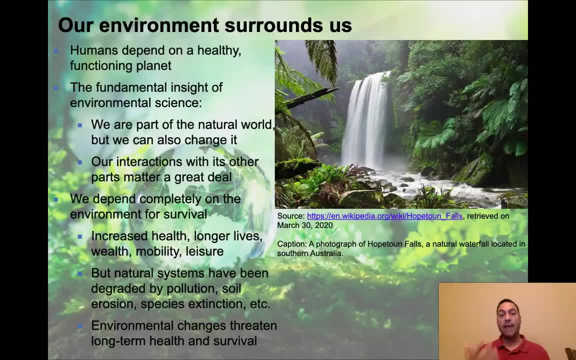 us alive and sustain us. Human beings are not capable of producing their own food. They have to derive their food from other sources. right, We can't go out and photosynthesize, for example, to produce food. We have to get it from the ecosystem. okay, So the fundamental insight. 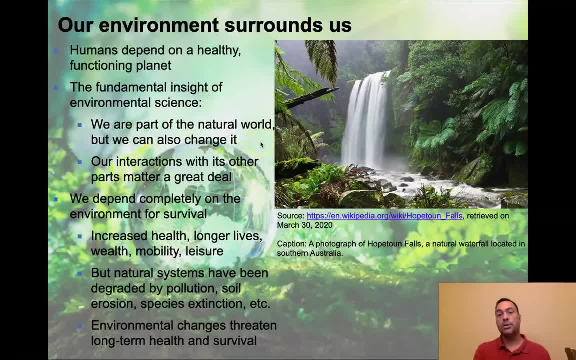 of environmental science is: we are part of the natural world, but we can also change it, and our interactions with it is with its other parts, matter a great deal. In fact, it's our imprint on those other parts. If we stress them too much, we can break them. 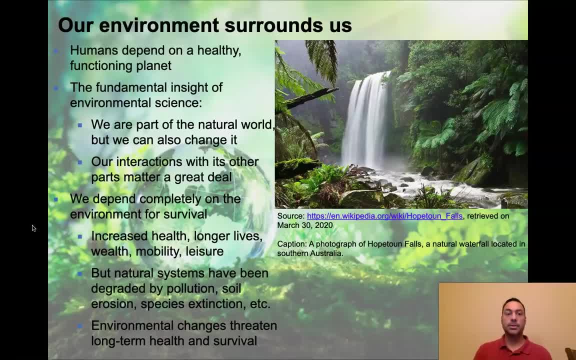 and if we break those relationships we can lose those relationships. So again, we depend completely on the environment for survival, We need it for increased health, We use it for longer lives, wealth, mobility, leisure, of course. But natural systems have. 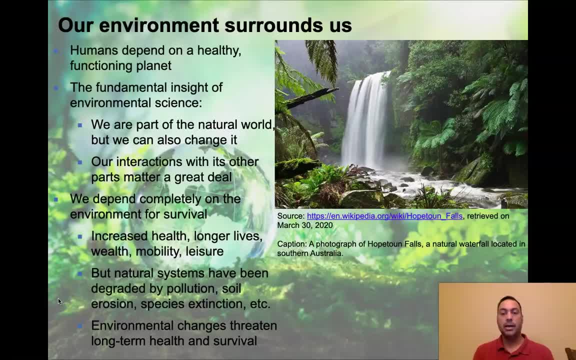 been degraded by pollution, soil erosion, species extinction, and the list goes on and on. In fact, we're going to cover a lot of these things later on in the course. Environmental change definitely threatens the long-term health and survival of portions of these ecosystems, which could eventually affect us. We ultimately rely on something. 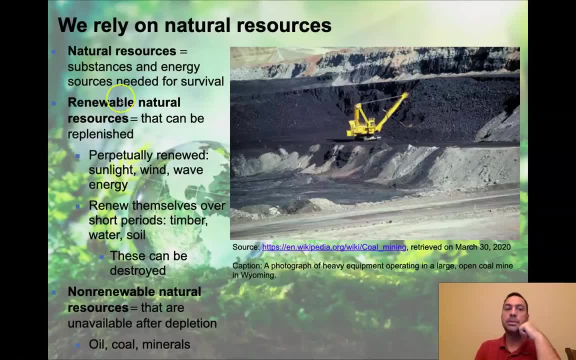 called natural resources. Now, natural resources are the substances of energy sources needed for survival. They come in different forms, but sometimes they're really obvious to us. For example, a natural resource that is really important to us is something like fruit right. 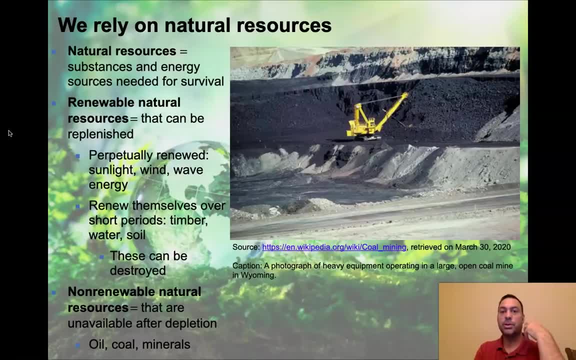 We can get off trees, That gives us the energy source that we need for survival. Of course, fruit comes from the photo or gets its energy from the photosynthesis carried out by the tree that produces that fruit. So the fact that we can get, say, apples off of an apple tree every year- 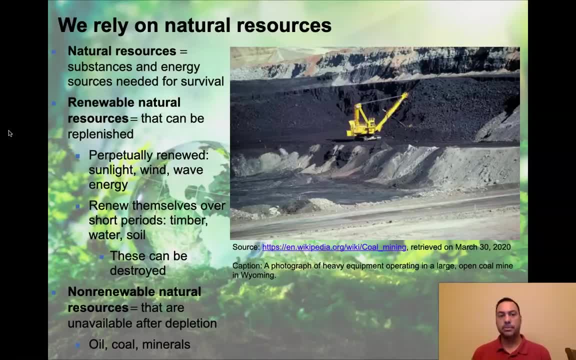 and use that energy internally makes it a renewable resource okay, Because we can do it every single year and the tree just does it automatically. So a renewable natural resource is something that can be replenished. It's perpetually renewable. It's something that 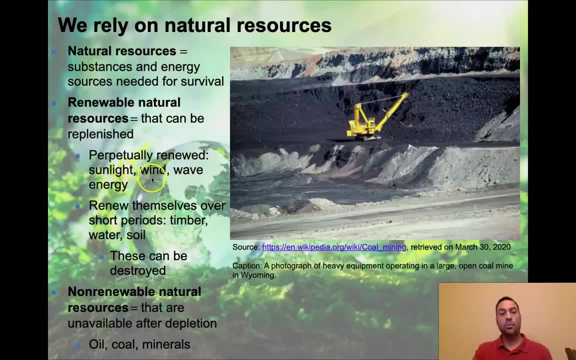 can be used for food And ultimately, that energy is coming from sunlight, wind or wave energy, And in fact wind and wave energy are also derived largely from sunlight as well. We may perhaps later on in the lecture series get into how that happens. I'm debating on how I'm going to take 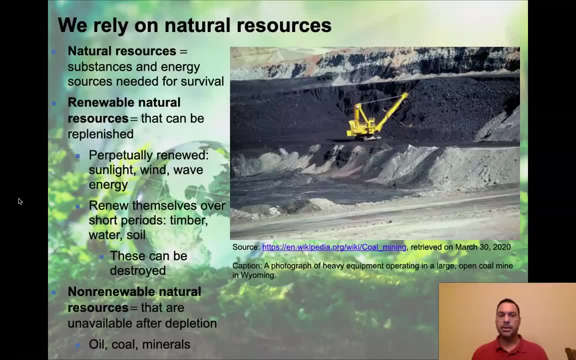 this course. But sunlight is a big deal And of course, that's what the tree is doing- is taking sunlight, taking that energy and transferring it to the apple, which is then transferred to us. Or if you look at the tree itself, you can see that the tree itself can renew themselves over short. 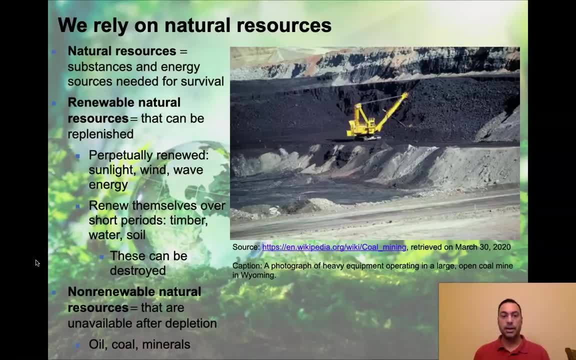 periods of time. Timber, water and soil- all can renew themselves over relatively short periods of times, But if you do it in such a way that you stress it so strongly, you can ultimately destroy these resources. You can in fact destroy the soil so it is no longer productive. You can, in 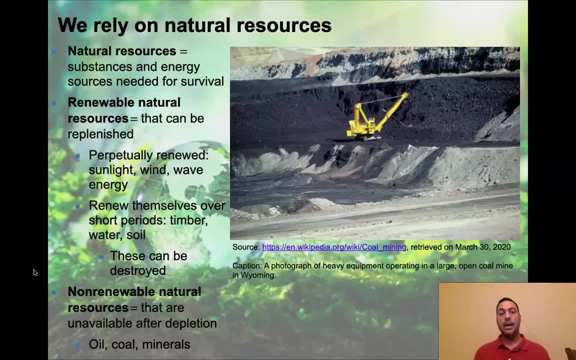 fact destroy a forest, so it is no longer going to return back in that original form and give us those same services it gave us before. In contrast, are non-renewable natural resources. These are the things that are available, that are unavailable after depletion. This includes oil. 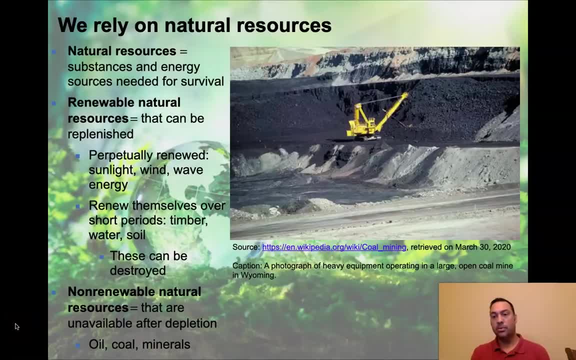 coal, minerals, landscape- If you stress it too much, you'll lose it- Things like this. And so here's an example of a non-renewable resource. This is a coal mine. This is actually a very, very, very large piece of heavy equipment operating in a large open pit coal mine in Wyoming in the 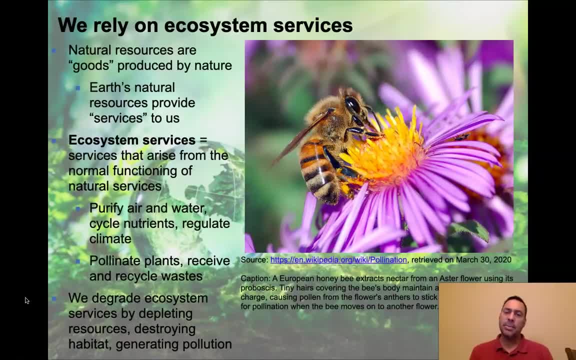 United States. Alright, so I mentioned the words ecosystem services before. Here it is again Ecosystem services. Natural resources are goods produced by nature. Earth's natural resources provide services to us, And so those services, or those ecosystem services, are services that arise from the normal. 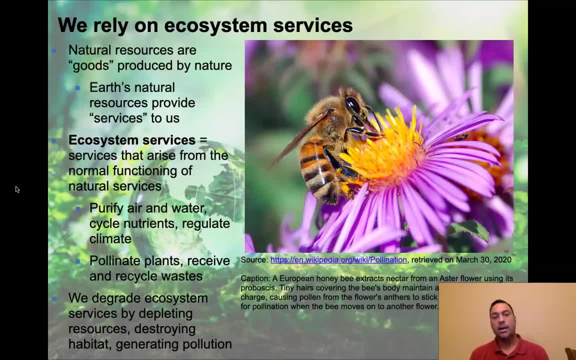 functioning of natural services. They purify the air and the water, They cycle nutrients, They regulate climate. We haven't talked about the processes yet. We're going to get into that a little bit later on- how the air is actually purified, how the water is purified. 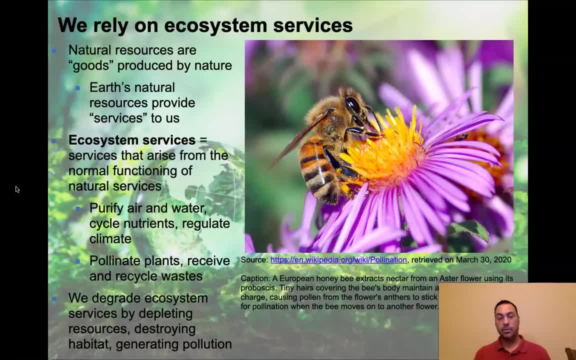 how nutrients are circulated throughout the geosphere, in fact, as well as through soils and things like this. But they also pollinate plants. We're going to get into what pollination is a little bit later on. Pollination is a really, really important part of the ecosystem. It's an 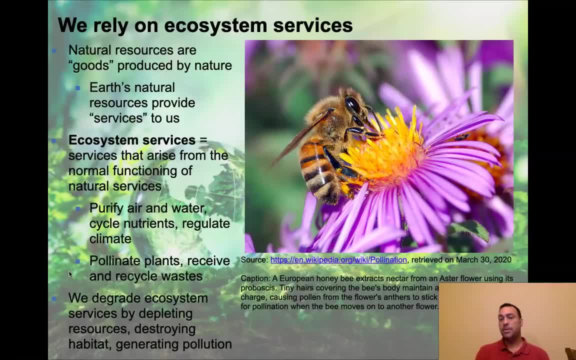 ecosystem service that is extremely crucial, Not just to humans, but to all of the other plants around us. They receive and recycle waste. Now we degrade ecosystem services by depleting the resources and by destroying their habitat and generating pollution. So this is an example of a pollinating 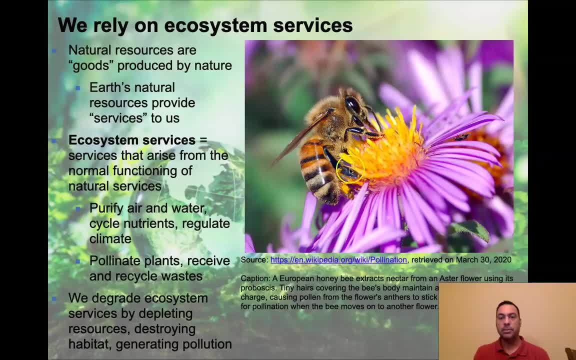 honeybee, If you look at it very closely. in this image there's little bits of pollen that are stuck to this bee, And when this bee goes from flower to flower it's going to transfer that pollen to other flowers And in return, the flower rewards the bee with something called nectar. 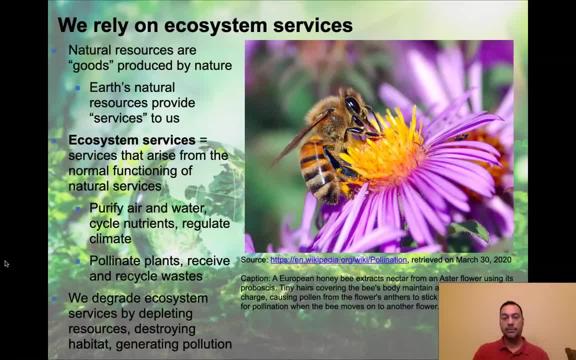 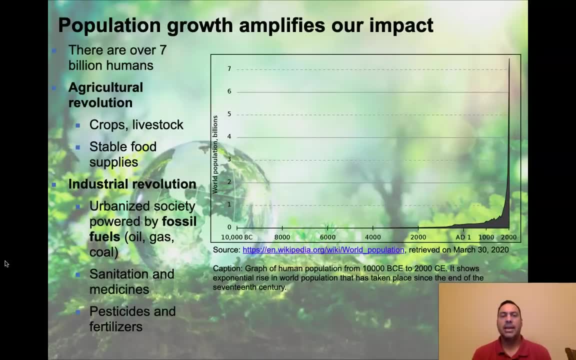 which has been used to create nectar Honey back at the hive. Now, in terms of how the population is interacting with this system, it's kind of important to know what do we mean by the population? Well, as of the time of the recording of this video, 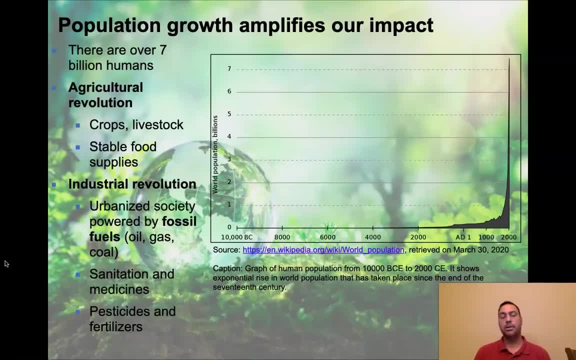 in early April 2020, there are over 7 billion humans- Almost 8 billion at this time. A large amount of that was brought about by something called the agricultural revolution. We have pretty stable food supplies right now. This has not always been. 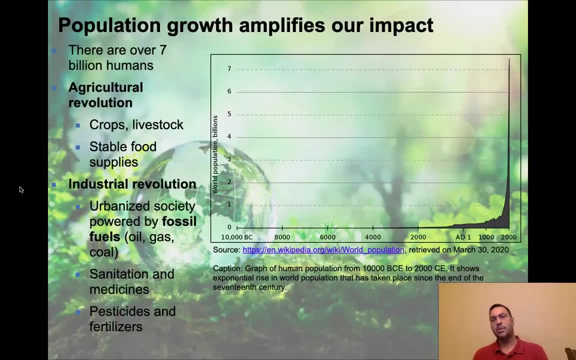 the case in human history. Human history is punctuated by times of famine and want and need and war and pestilence. And the pestilence isn't always on us. Sometimes it's on a crop. The potato famine in Ireland, for example, is a classic example of this. Ultimately, a lot of this is 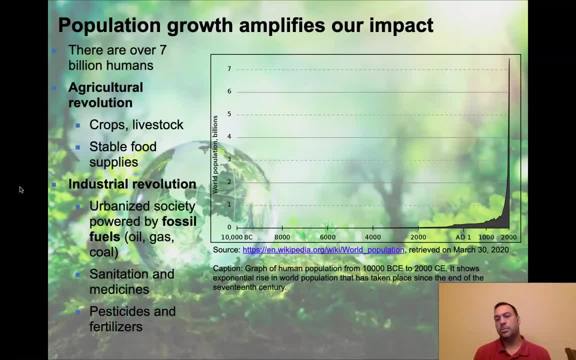 derived from something called the industrial revolution, which took place in the period of time after the 1700s, With the 1700s on, Urbanized society, powered by fossil fuels- oil, gas and coal- And actually in the early form there was even whales that they used to hunt. They used to use whale oil. 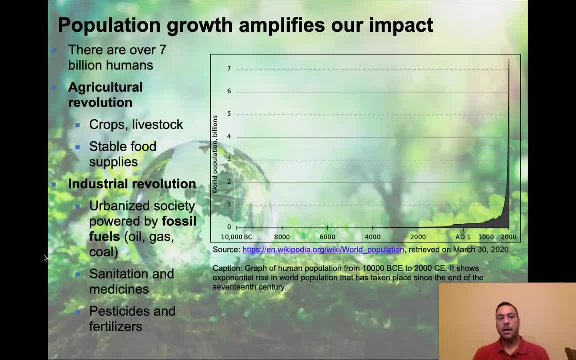 to be able to power this urbanized society. We improved sanitation and medicines right, And, of course, with better sanitation and better medicine, you're able to have a healthier lifestyle. And then pesticides and fertilizers were used, which made it easier to grow things. 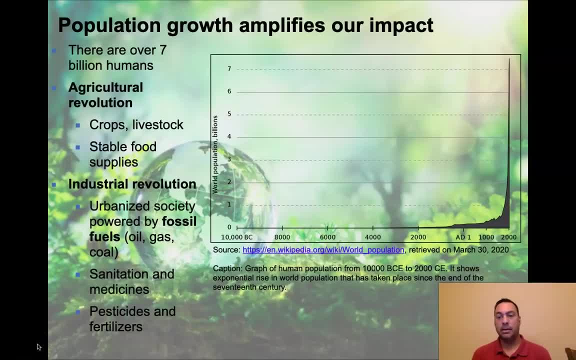 and to take care of things without pests coming in And attacking what it is that you're trying to produce And, as a consequence we could actually see. this is the population growth of human beings from 10,000 BC all the way to the year 2000 in the 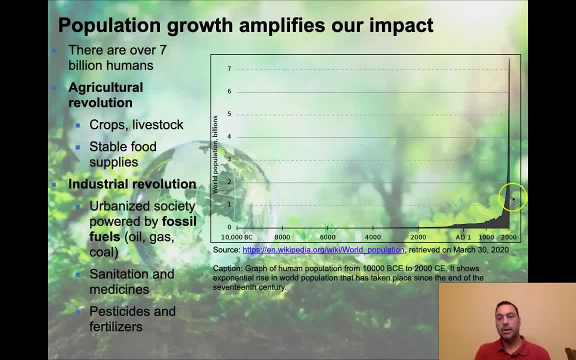 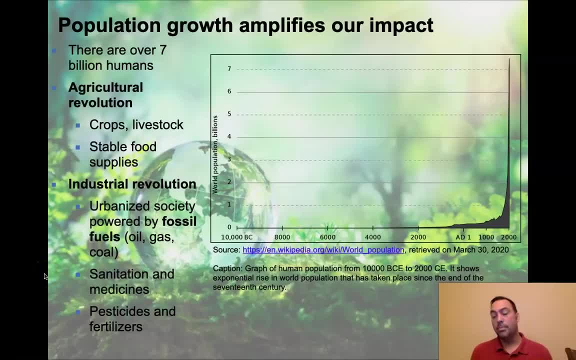 revolution, that agricultural revolution, that agricultural revolution, that agricultural revolution That's allowed that to happen, And that number of people is still going up And we really don't know how high it's going to go, But it's going to be quite a large number, And so a 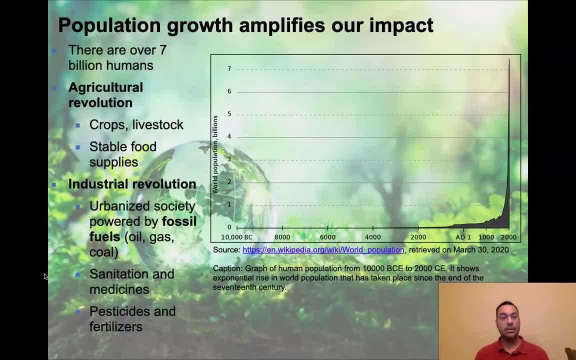 lot of these people are going to require these services: sanitation, medicine, going to need stable food supplies. They're going to be desiring farming, In addition to the comforts of having televisions and air conditioning and washing machines and dishwashers and things like. 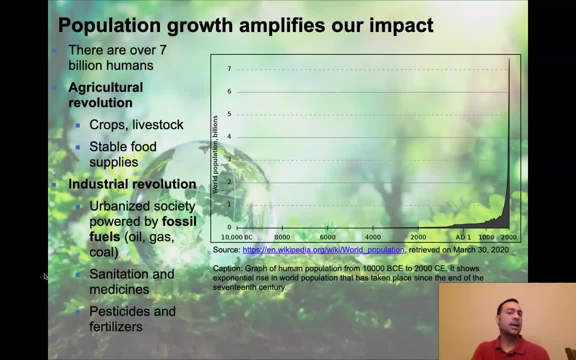 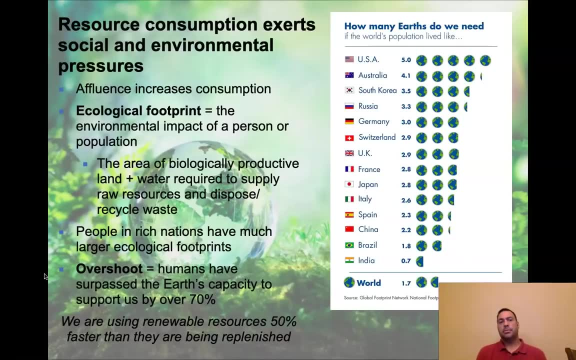 this. So there's a lot of stuff that's headed our way. The question this is: can the earth accommodate? accommodate all of that? How will it accommodate all of these things? So resource consumption exerts social and environmental pressures. This is an 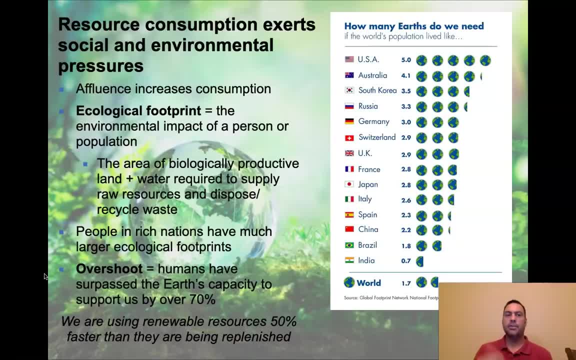 interesting little graphic that we have here. First off, affluence increases consumption. The more affluent you are, the more stuff you consume, Whether it be you know, and some things, by the way, aren't equal to other things. So for 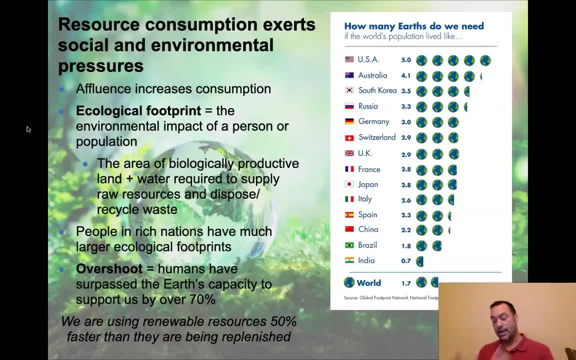 example, if you consume a lot of celery, that's a lot different than if you consume a lot of steak. even if it's a pound of each Steak is a lot more expensive. It takes a lot more energy and a lot more resources to produce it, And 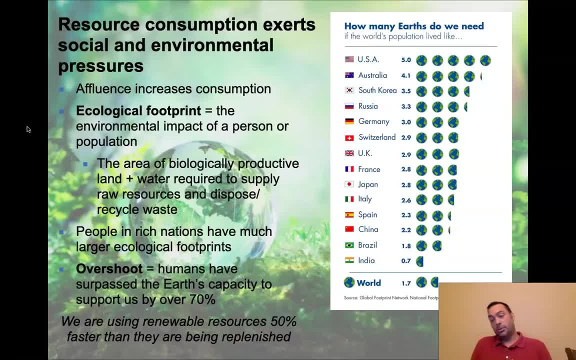 you generally have to be more affluent to be able to consume or to purchase a pound of steak versus a pound of celery. So as a consequence, we see that that tends to happen. We're going to get into that later on, But as people get, 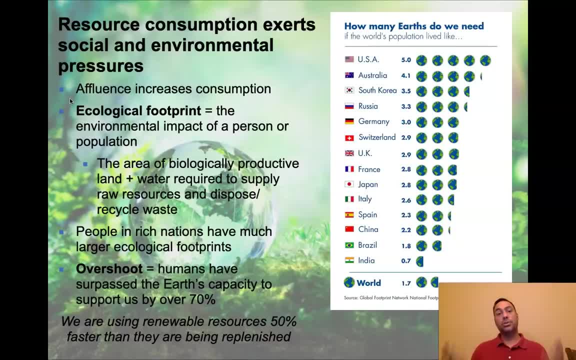 wealthier, they tend to eat more expensive things that require more resources to produce. So affluence increases consumption And that results in something called the ecological footprint. The environmental impact of a person or population usually is measured in a land area right. So this is the area. 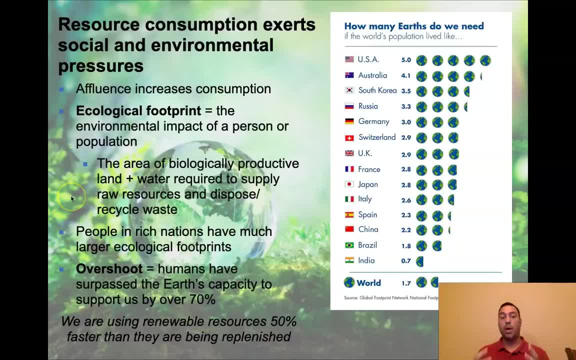 of biologically productive land plus water. So it's the amount of land required to supply raw resources and dispose of it, slash, recycle waste. In other words, it's the amount of land used to keep you alive, given the average consumption of human beings in that area right. 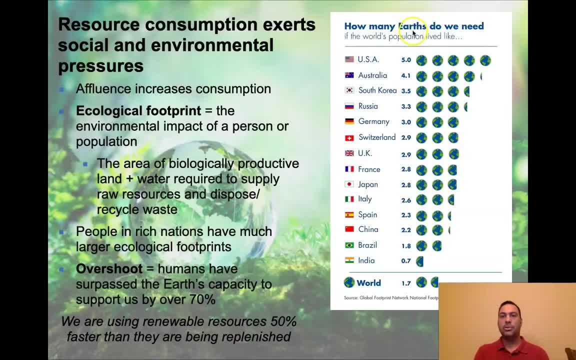 So let's give you an example of this over here. How many earths do we need if the world's population lived like, let's say, the United States of America where this is being recorded? So USA, it turns out, if we all- all seven, almost. 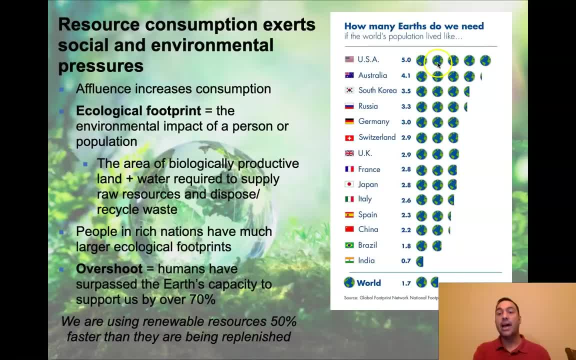 eight billion of us live just like the way that Americans live. it would require five earths of resources to be able to accommodate that, Whereas on the flip side of that, if everybody lived just like India does, it would only require seven tenths of one Earth. And we notice that as we go from India to 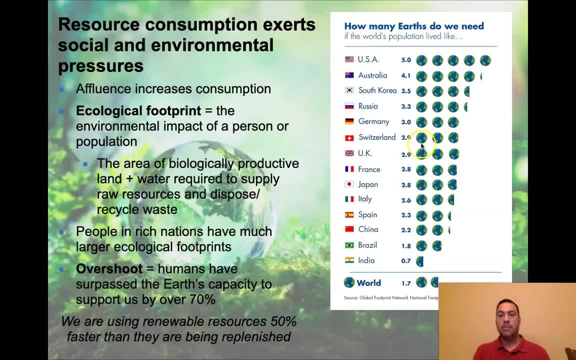 Brazil, to China, to Spain. as we head up this chart, these are much more affluent countries as you go towards the top. South Korea, Australia, Russia is kind of an interesting case. Germany and Switzerland are, of course, very affluent countries, as well as the UK, France, Japan, So we could see this very interesting. 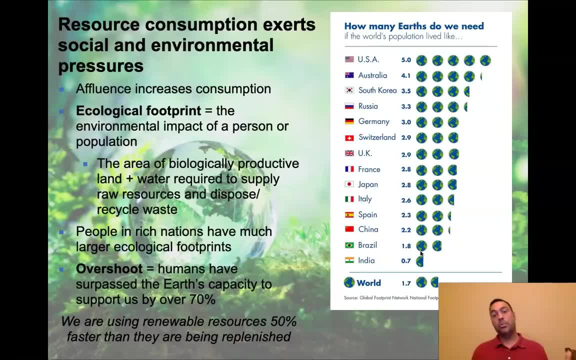 trend between affluence, and how many Earths would be required for everybody to live, just like everybody in that country? Currently, the world is at 1.7 Earths, And so that should drive a pretty interesting question to your mind. If there's one Earth and everybody's on it and we're- 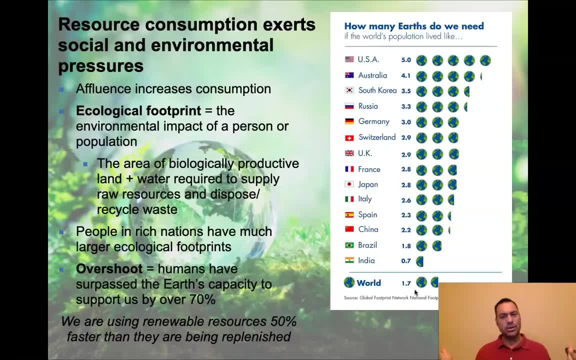 growing in population. then how is it we require 1.7 Earths of resources to make that happen. We're going to get into how that happens a little bit later on, But the concept of that, of going above and beyond your ecosystem, is a little bit different than what we're used to seeing in the 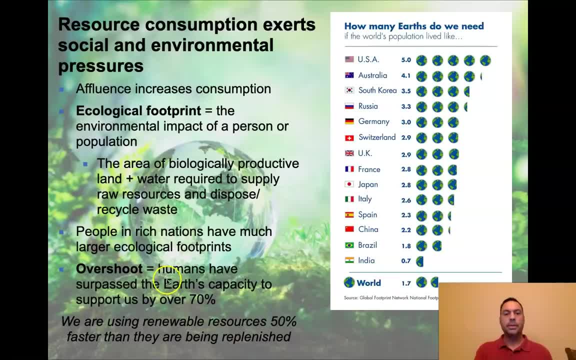 world. So we're going to get into that a little bit later on. But the concept of that, of going above and beyond your ecosystem, is a little bit different than what we're used to seeing in. the footprint is called overshoot. These are humans have surpassed the Earth's. 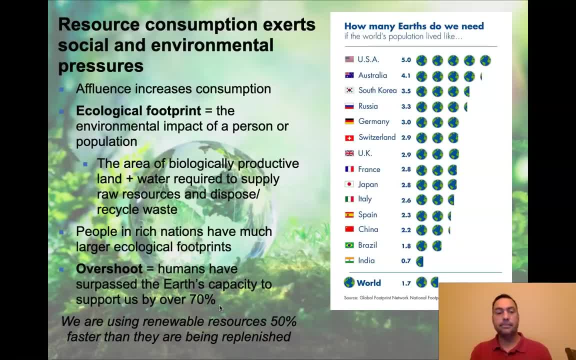 capacity to support us by over 70%. We are using renewable resources 50% faster than they are being replenished. So basically, we have a problem. What we're consuming doesn't match what the Earth is providing naturally, So there's a subsidy coming in from some location in the ecosystem We're going to talk about. 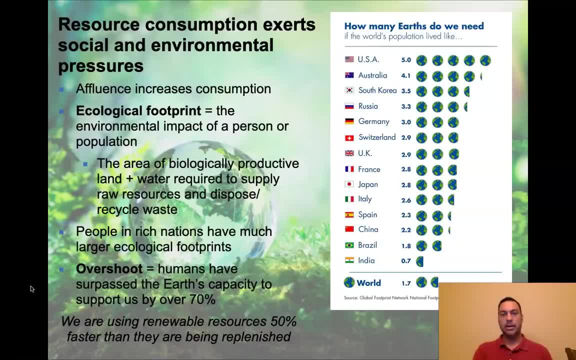 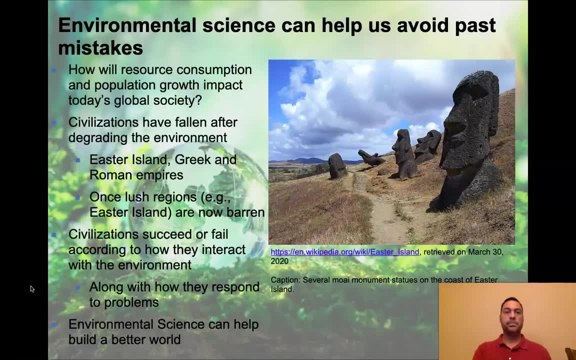 what that subsidy is and where it's coming from a little bit later on in another lecture. But just be kind of aware that we are definitely in an overshoot situation currently on Earth. Now, understanding what environmental science is and how to apply it can help. 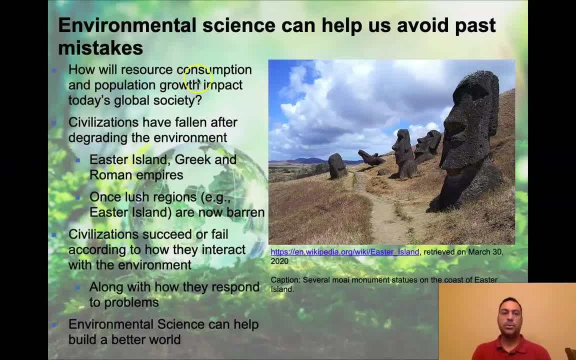 us avoid past mistakes. So how will resource consumption and population growth impact today's global society? Right, We're growing. What is the impact going to be? How is it going to change things? How do we decide how to allocate what resources in the directions that we want them to go? 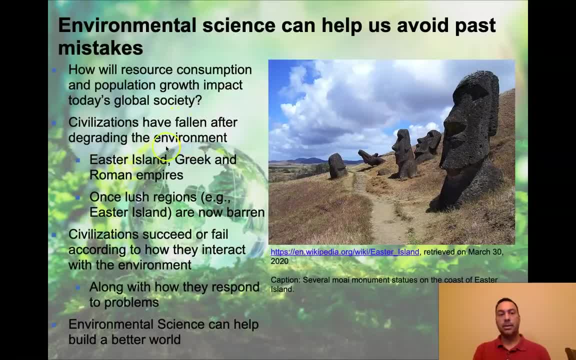 Civilizations have fallen after degrading the environment. This is not the kind of some benign concern. It happens. It's happened on smaller scales and now people are starting to look at a more global scale. So Easter Island, which is located in the East Pacific off the coast of South America, is a 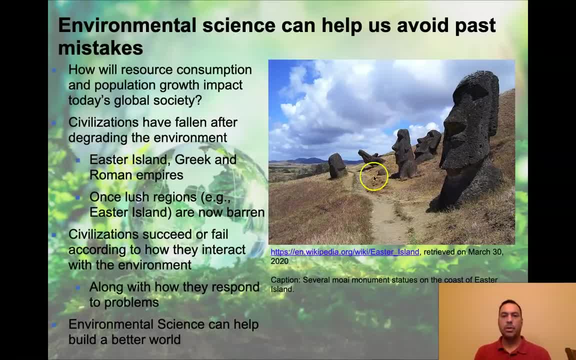 classic example of this. This is where we see what used to be a lush forested area. The lush forested area has been completely decimated, But a lot of it is believed to have been. a lot of those resources were believed to have been used to erect these monumental statues that they have all over I mean. 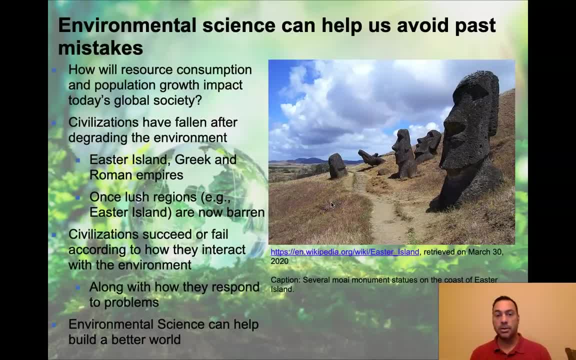 the island is famous for them, But the amount of resources it took to probably put those in place wound up costing them their entire forests, and their forest ecosystem collapsed, and their populations probably collapsed as well. Of course, you can read a lot about Easter Island. It's a very famous case. So this one very lush area. 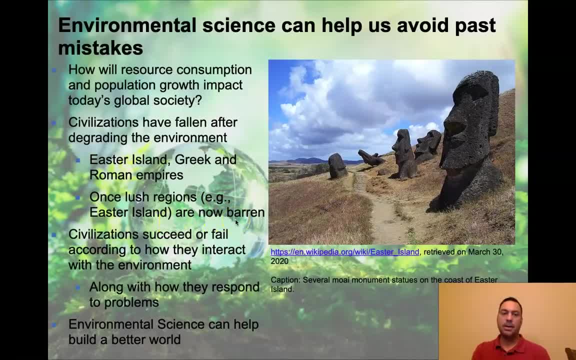 Easter Island, for example, is now barren, But it's happened in other places too. It happened in the Greek and Roman empires. Some people have said that it happened at Carthage as well, So there's a lot of information that suggests that. 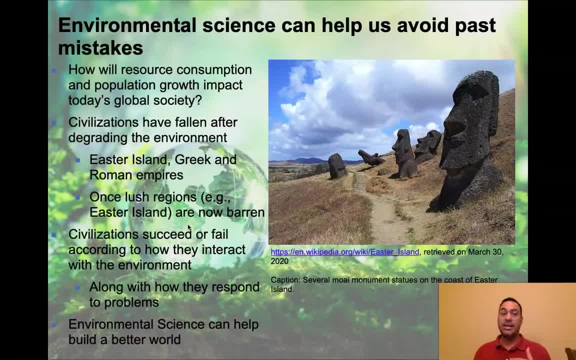 understanding environmental science can help us avoid some type of very negative fate that we can't see coming. In fact, when I'm recording this right now, the COVID-19 virus is currently moving across the planet. It's possible that it will be solved in a very short period of time, or it could persist for a very long period of. 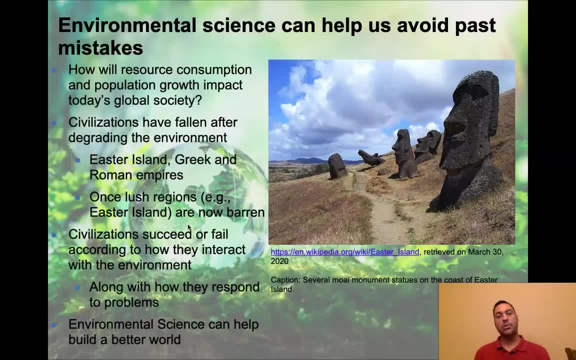 time, But understanding environmental science lets us know that. you know, when we're dealing with something like this, it's probably best to stay indoors, to stay safe and to stay away from these things. That's science telling us from experience what might work. 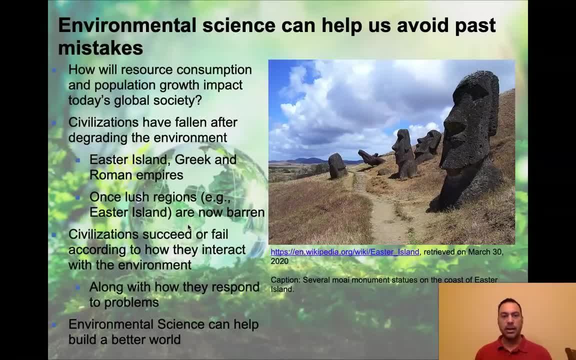 for the future, And we're going to get into how science works here briefly in a couple of slides. So civilizations succeed or fail according to how they interact with the environment, along with how they respond to problems. Subtitles by the Amaraorg community. 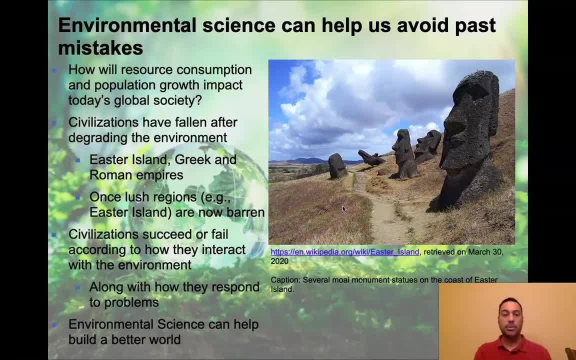 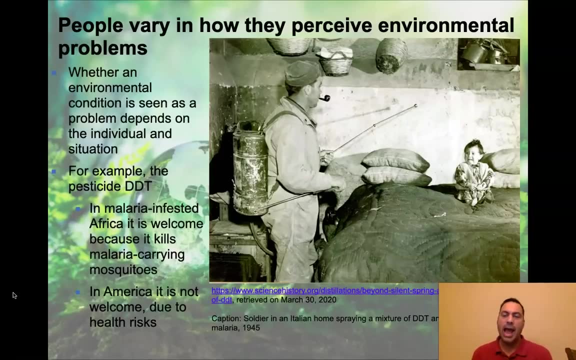 So, in this situation, they cut down all the trees, they weren't able to recover it and the civilization essentially collapsed. So environmental science can help build a better world. That's the hope, That's what we're hoping will happen going forward. Now, how do we go about solving these problems? How do we? 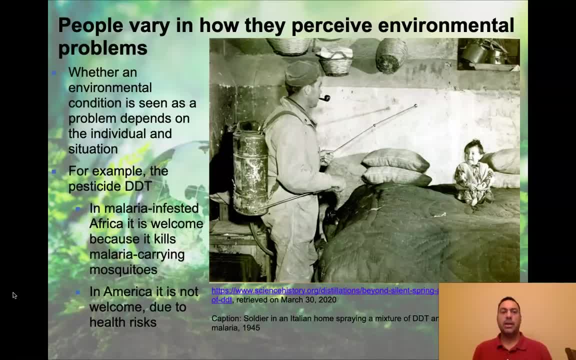 One of the biggest issues we have is how these problems are perceived and how our responses are perceived. So sometimes it's cultural. So whether an environment condition is seen as a problem depends on the individual and the situation Right. So a classic example of this is DDT. DDT is a compound that was used to deal with malaria. 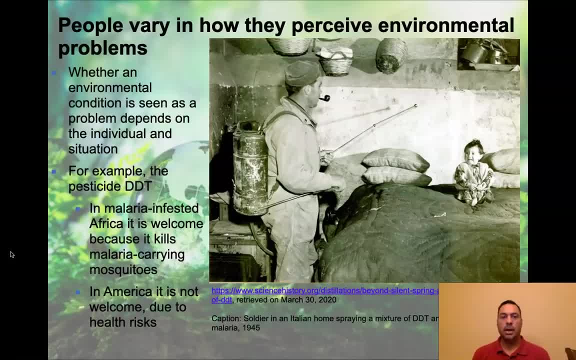 infestations across the world. In Africa it is welcome because it kills malaria-killing mosquitoes, But in America it is not welcome due to the health risks. So DDT is considered a very toxic thing to put on your kids, But in Africa they're not welcome because they're 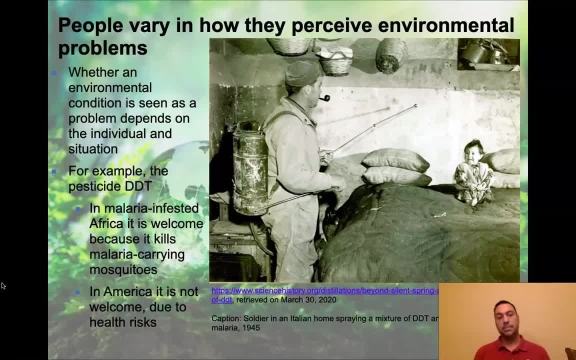 two of the biggest factors that they're affected by. In Africa, the fear is greater that you're going to be affected by something that's gonna give you malaria. Right, It's a cultural perception that we see here. What we see here in the image is: this is an Italian soldier in Italy spraying mixture of DDT. 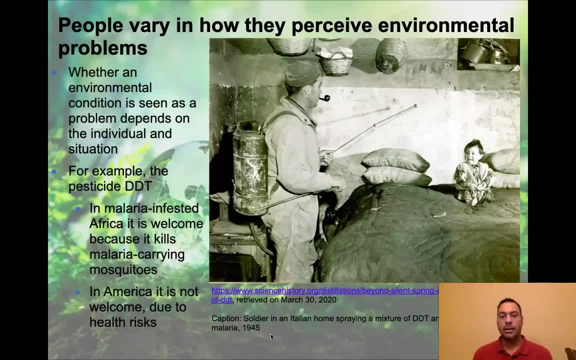 and kerosene to control malaria. And this is in war-torn Italy in 1945.. And you can see the child is not terribly happy with this development. Question is: would you be okay with DDT being sprayed on you or your children? If you lived in the United States it would. 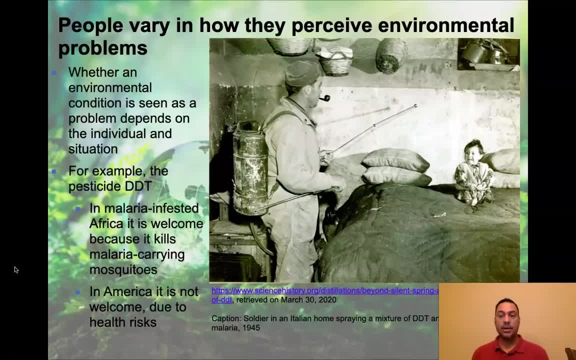 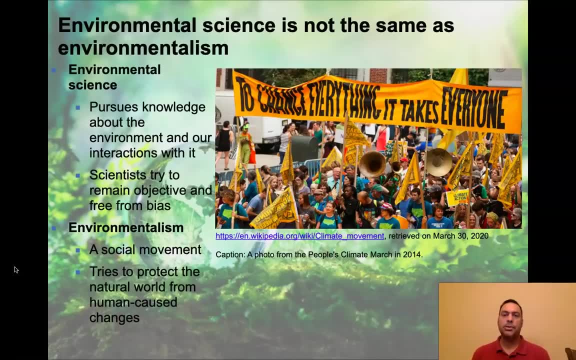 probably be perceived as a very bad thing. If you lived in Africa, it probably wouldn't be considered such a big deal. Now I want to make sure that, as we go forward, that we understand there's a difference between what environmental science is and what it isn't, And one of 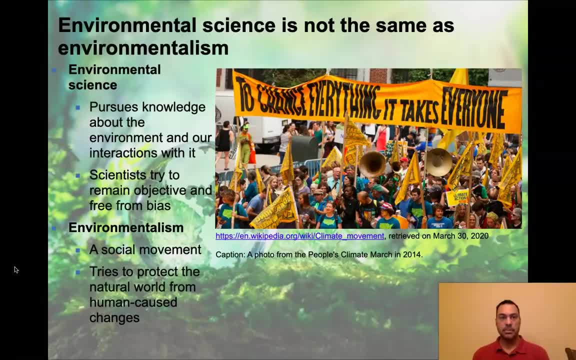 the things that is constantly conflated with is environmentalism, So let's talk about what environmental science is. So environmental science pursues knowledge about the environment and our interactions with it. Scientists try to remain objective and free from bias. Okay, so whatever the data says, it says: 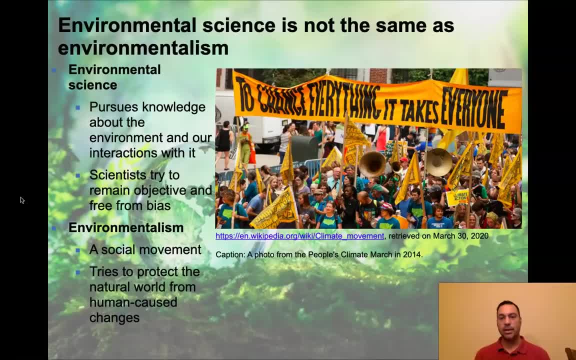 we need to work with it. We can't massage things, We can't change things. We need to work with what we have. This is a little different than from a little different than other things that you might see going on in the world. Another. 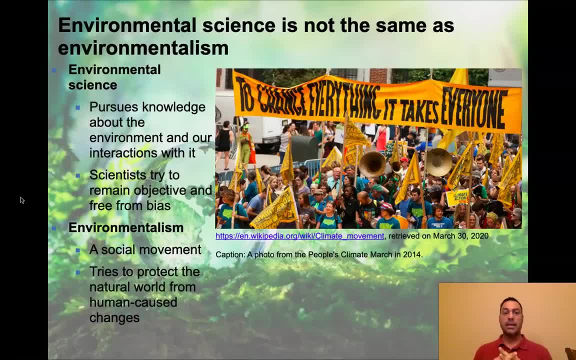 thing you might see that's a little different than other things that you might see going on in the world. Another thing that you might see that's constantly conflated with environmental science is environmentalism. Environmentalism is a social movement. Sometimes it's a political movement, but it's largely a social movement that tries to 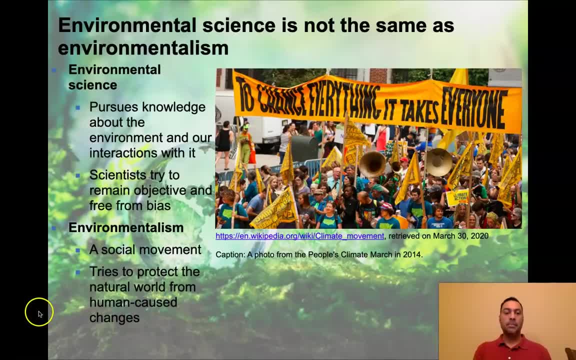 protect the natural world from human-caused changes. Now, environmentalism is not objective, It is not free from bias, It is very subjective, right? People that are usually in the environmentalism or environmentalist movements have a very, very strong opinion about a certain way that either. 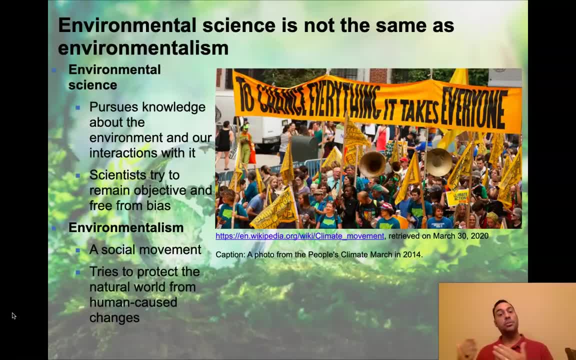 society should go or a certain way that a problem should be dealt with. Scientists and the social scientists can be environmentalists, right, And environmentalists can be scientists, but they are actually different spheres of thinking, As long as you understand that one is a series of actions, or let's say it's a social movement and the other one is an. 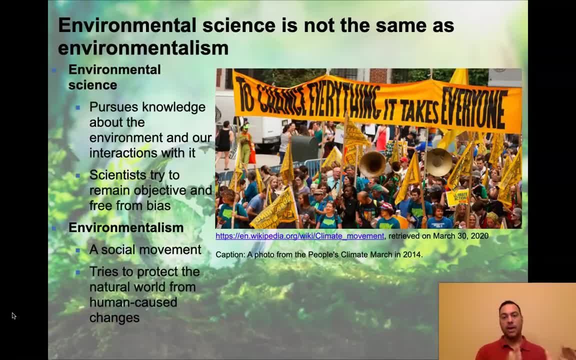 actual movement, it's a social movement And the other one is a social movement, objective form of looking at the environment of the world in which we live. then you're kind of going to be okay going forward. If you're kind of confused about that kind of stuff, you're going to. 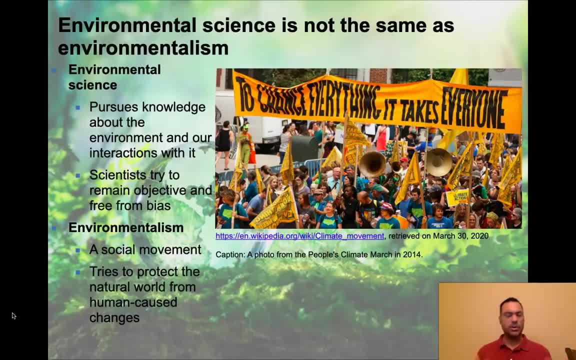 get stuck on the wait a minute. I thought this class was about saving the whales, or I thought this class was about Greenpeace. Hey, it's great to save whales. It's great to study what goes on with Greenpeace. It's great to study what's happening with those things, What might be. 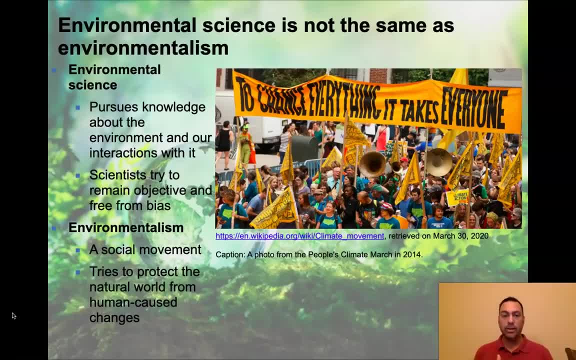 driving that environmentalism in Greenpeace or in saving whales. Might be environmental science knowledge behind that, but just be aware that those are organizations that are a social movement, And so you can typically recognize a social movement when you see, you know, people marching down the road. This is from the. 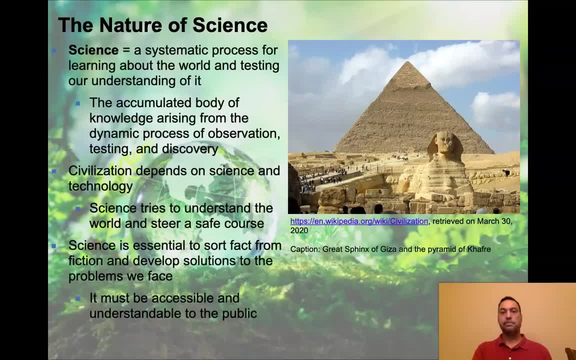 People's Climate March in 2014.. So that, of course, leaves us with the question of what is science? So we're not going to get into a deep discussion what science is just in this little lecture, But we are going to kind of give you a very brief introduction to the concept of what it is. 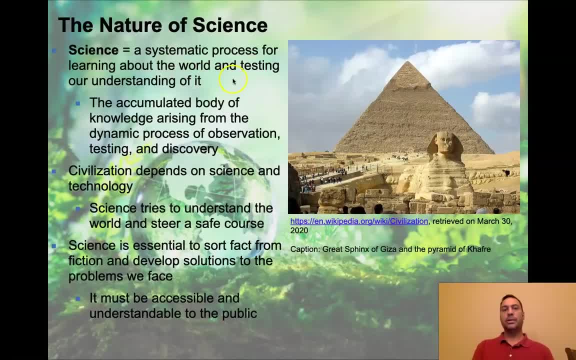 So science is a systematic process for learning about the world and testing our understanding of it, The accumulated body of knowledge arising from the dynamic processes or process of observation, testing and discovery. Civilization depends upon science, and technology just has, in order to move forward Our interactions with each other, our ability to observe. 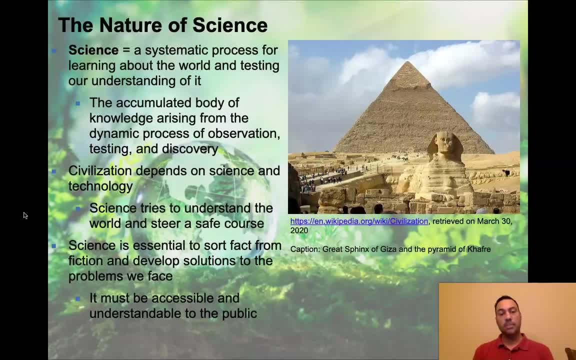 test, discover and to trade those ideas with each other is fundamental to how society operates. Science tries to understand the world and steer a safe course. That's our ultimate goal. right, If you know, for example, like I mentioned earlier, we have this virus. If you know that there's a virus, 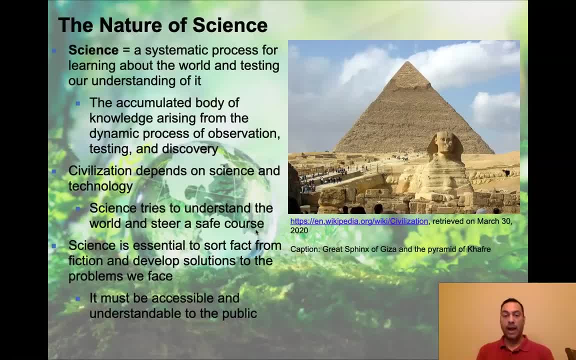 that's raging across the world and that virus has fatal impacts on certain groups of people or even on the entire population. it's best to stay steered or to steer away from it, And that's what we're going to do. We're going to steer clear of that virus, right? How do we know to do that Past? 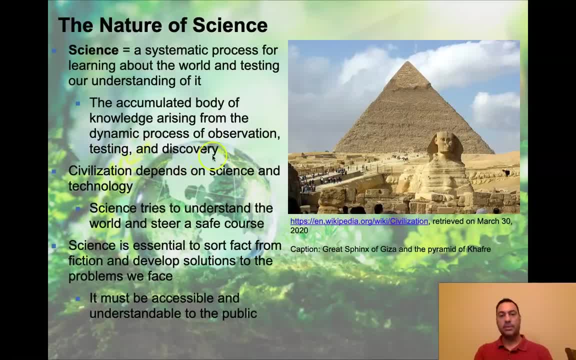 experience right. We've observed it, We've tested it. We've discovered that staying away from the virus keeps us safe, And then we don't die of it. Has that always been kind of common sense? No, It used to be very, very different. People used to die left and right from these types of viruses. 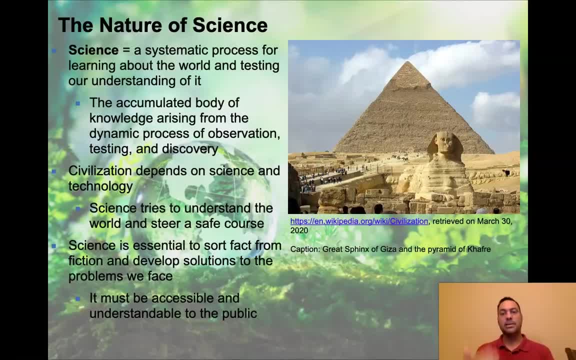 in human history And our understanding of how these things operate have informed us in our proper responses. Now, science is essential to sort fact from fiction and develop solutions to the problems we face. And that's just how it is. I mean, it's designed to figure out what is. 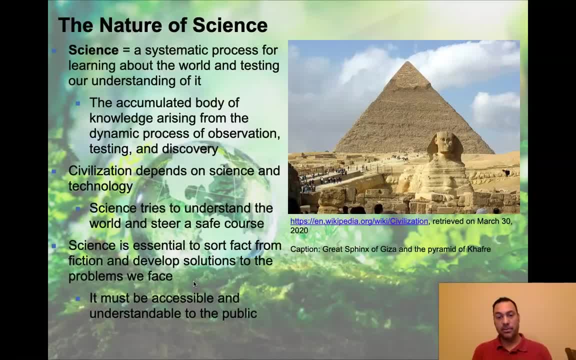 the truth about a certain thing, to the best of our ability to find it. Sometimes the truth is knowing what it isn't right. We don't know what a solution is, but we know that these aren't solutions, right. So sometimes science is in the negative right. This is what we know. 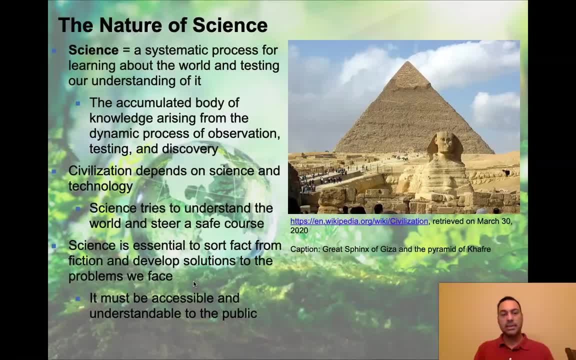 to do if there's ever this problem, And so that's what science does. It must be accessible and understandable to the public, And that's really where you're kind of coming into. my lecture is: I'm trying to find a way and I'm gonna work. 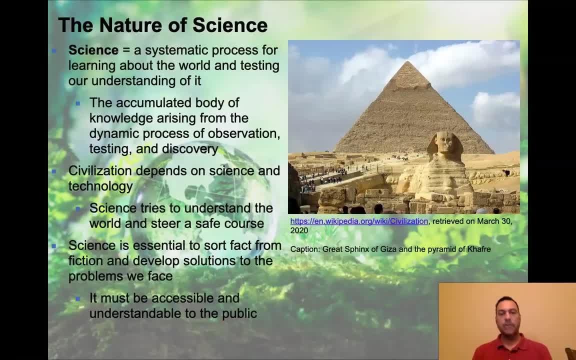 really hard at it over the next series of lectures that we put out, to make this information accessible and understandable, And that includes understanding things like the vocabulary. I'm going to emphasize the vocabulary very strongly. You're gonna find that any freshman level or sophomore level- 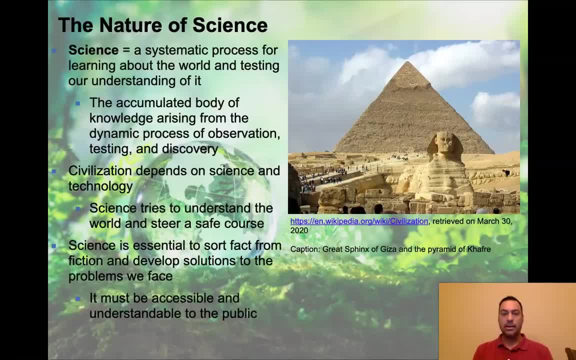 class is going to emphasize the vocabulary because without it you're gonna be lost in any conversations or any reading that you ever do on the topic. Okay, in terms of the kinds of science that we've done, you know we have the Great Pyramid, here's the Sphinx, out here in the front and, of course, the 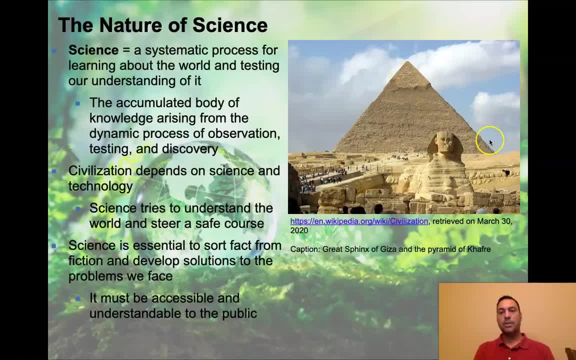 ability to construct something like this required some previous experience. right, This is something that they observed, they tested, they actually had some engineering knowledge on. they went out and they built the Great Pyramid. The same thing with the Sphinx- right The artist that came through and 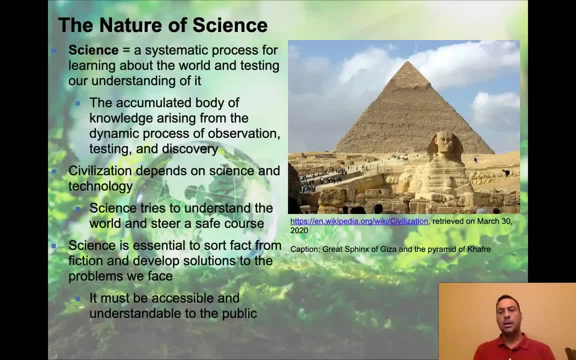 carved out this thing, and I believe it's in sandstone. I might be wrong, but whoever did this had a tremendous amount of experience, And so we recognize that, that this requires a certain level of sophistication that science brings that civilization ultimately depends upon, And when we look at these things, we 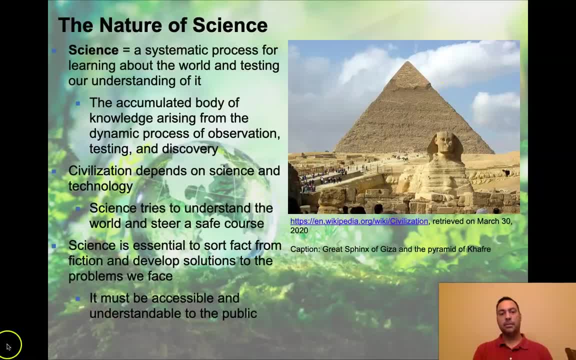 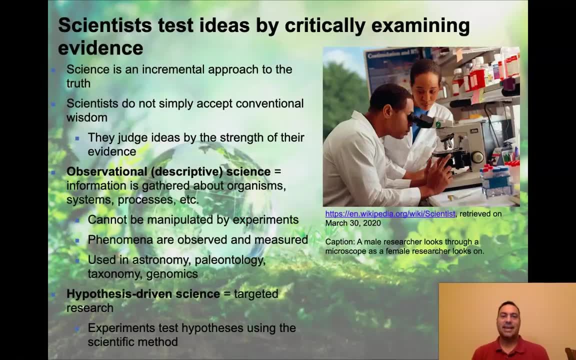 recognize these as major, as major symbols of the ancient Egyptian civilization. Now scientists test ideas by critically examining evidence. Now, science is an incremental approach to the truth. In other words, we don't usually figure out what the answer is the very first time. 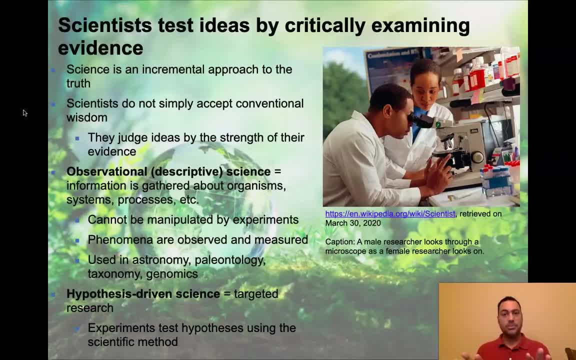 Sometimes, again, there might be a thousand different options on what we're looking at. There might be a thousand different explanations for a phenomenon, And sometimes we just simply say: not that one, not that one, not that one, right, So we incrementally approach it. okay. Now the other thing is that 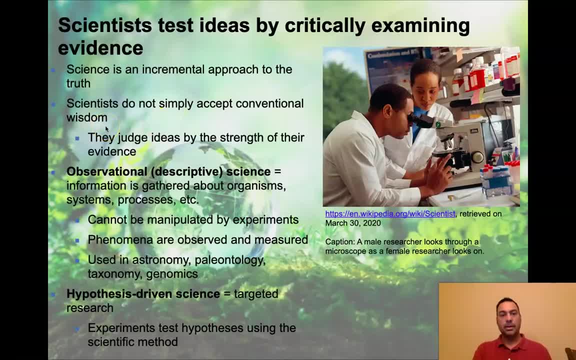 scientists do not simply accept conventional wisdom. They judge ideas by the strength of their evidence. And we will find as we go forward in the class that a lot of the things that people take for granted just simply aren't true. And I don't want to tip my hand on some of these conversations, but some of the 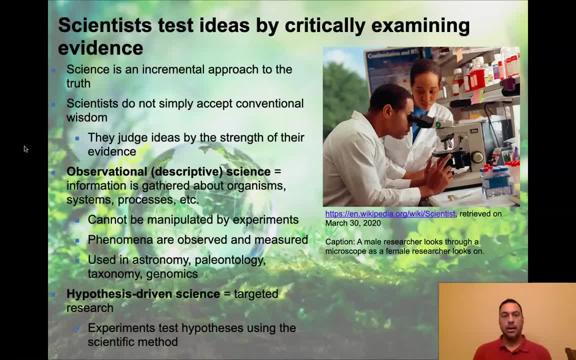 issues such as how to carry out proper agriculture, for example, that conventional knowledge that you might have been raised with. it's not just a simply wrong, And we're going to talk about that a little bit later on. Now there's two different ways we carry out science. There's 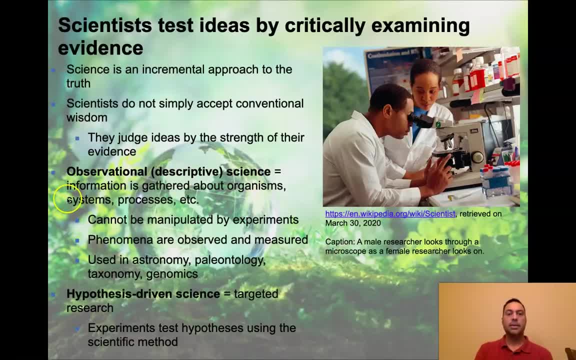 observational or descriptive science. This is information carried or gathered about organisms, systems, processes, whatever that cannot be manipulated by experiments. all right, The phenomena are observed and measured. It's used in astronomy, paleontology, taxonomy, genomics. A great form of this is geology. 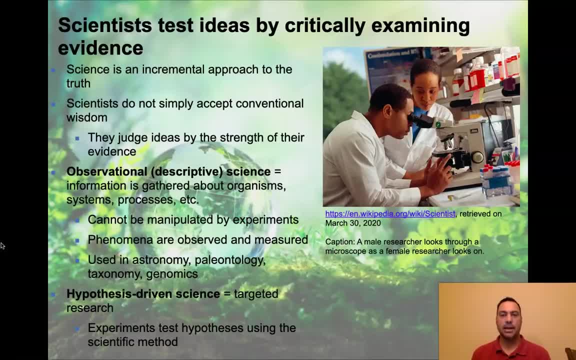 I actually have a background in geology. Imagine something as amazing as a volcano. A volcano is something that you can't really manipulate using an experiment. You can build models of volcanoes, but never, ever going to get to the actual heart of what happens in a volcano. You actually have to go out and 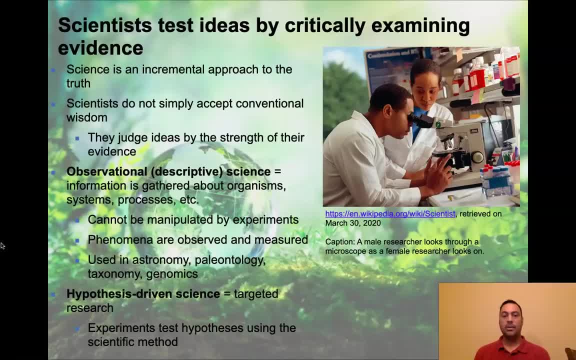 just simply watch these things using different ways. right, You might look at seismics, You might listen to the sounds that come out of it, You might be looking at the gases that come out of a volcano, right? But you're gonna be observing and 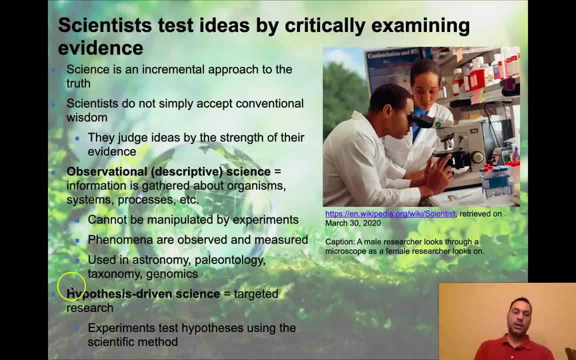 measuring a lot of stuff. In contrast with that is hypothesis-driven science. This is targeted research. This is where you're doing experiments, You're manipulating things and you're seeing what happens as a consequence of that manipulation. So these are experiments, test hypotheses using the scientific 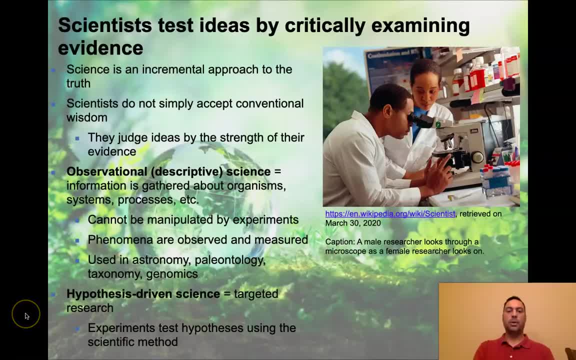 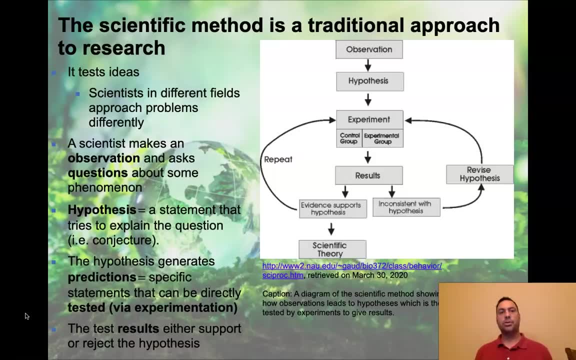 method. That word hypothesis is kind of a loaded word. We're gonna get into that here in a moment. All right, So this is the traditional approach for the scientific method. It's the traditional approach for the scientific method. You've heard, you probably have seen diagrams like this your entire life. 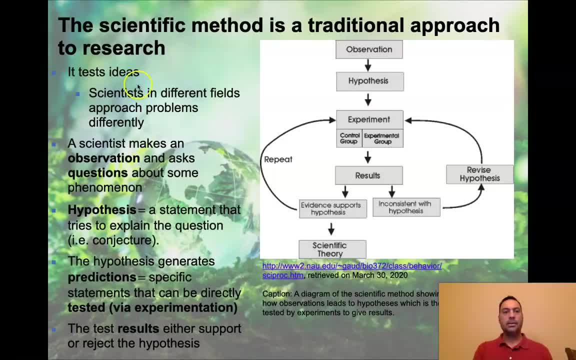 We're going to get into it here in a moment. Now. a scientific method tests ideas. Scientists in different fields approach problems differently. The way a geologist is going to look at a problem is going to be very different than the way a biologist or, in some cases, if you're dealing with the social sciences. 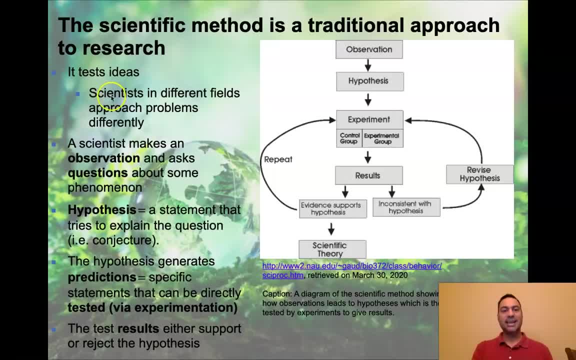 the way that they're going to approach the problems. okay, So a scientist makes an observation and asks questions about some phenomenon. This is how it always starts, right. So there's an observation, then there's the next problem that 있습니다. 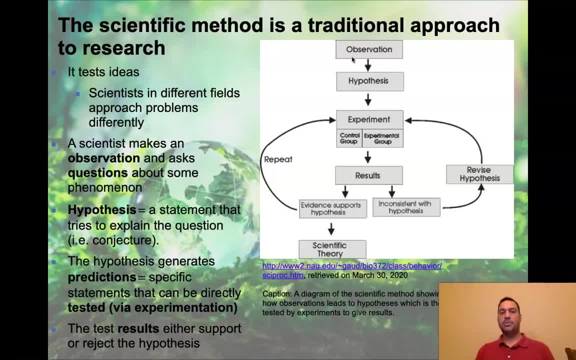 and then, and there's a question, For example, maybe the observation is: there's a very large valley in the middle of northern Arizona. How did it get? here might be the question. Okay, and if you, if you don't realize what I'm talking about, 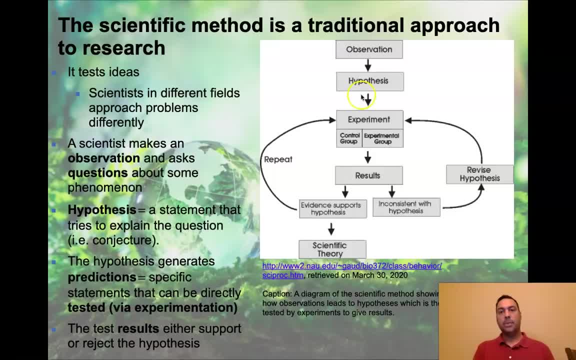 here or what I'm talking about here. I'm talking about the Grand Canyon, So there might be a hypothesis statement that tries to come to explain the question. The word hypothesis is kind of one of those weird loaded terms that you've probably heard your whole life and people say it's an educated guess. I've 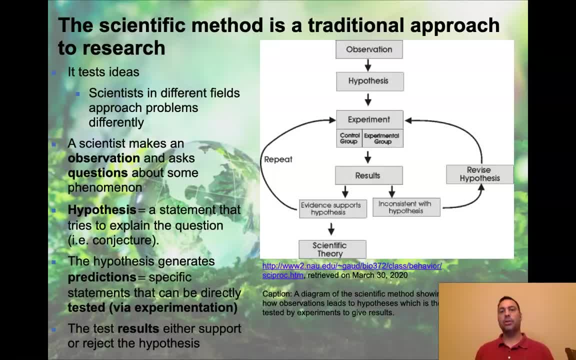 never really liked the word educated guess. It's really not a good interpretation of the word hypothesis. The closest word in English is the word conjecture, right, So conjecture is an understand, is a statement of under or statement of explanation. is based upon less than all the information. 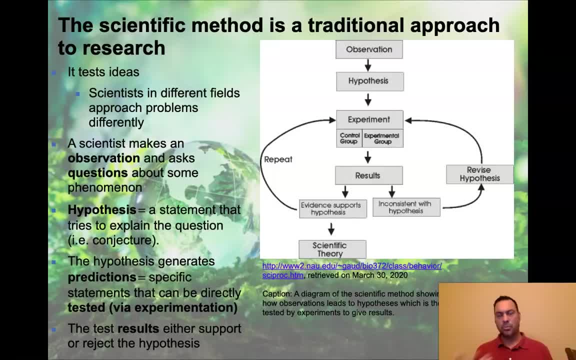 that might be available, especially going forward. So that's when we're talking about hypotheses. This is a conjecture, And so what you do is you take your hypothesis and you generate these predictions, and specific statements can then be tested through experimentation. So maybe, as you're looking at the Grand Canyon, you might. 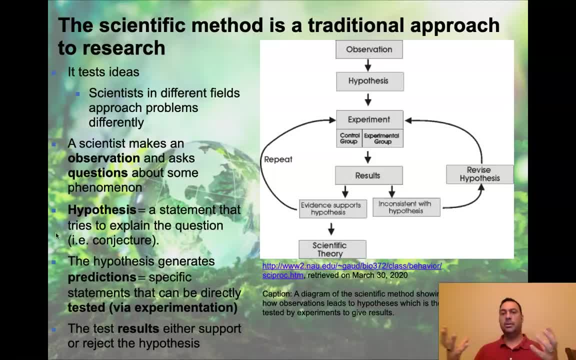 have several conjectures about how this giant, beautiful feature in northern Arizona formed. Maybe it was formed from a. maybe there's a volcano that's ripped open the area. Maybe a lava flow has covered the area and burned a giant hole down into the bottom. Maybe there's 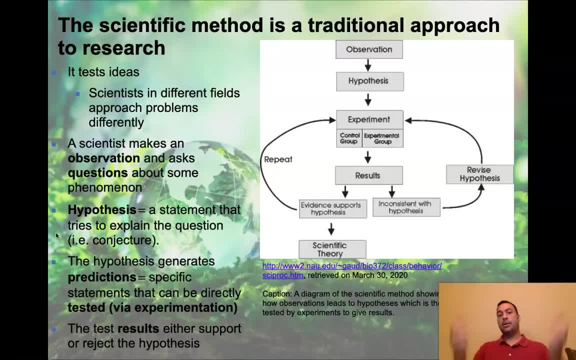 maybe it's a giant river valley that's caused when the entire plateau in northern Arizona uplifts. There's different ways of going about this and looking at the experiments, Ok, So we would carry out these experimentations, We would get results. So maybe as I go out into the Grand Canyon, I realize while 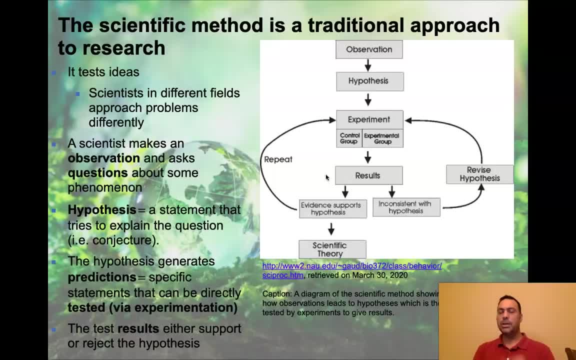 there are lava flows. there are very few of them and they don't seem to really control the location of where the Valley is. In fact, the Valley seems, if anything, to have captured something- these lava flows- in some interesting ways. So maybe it's not created by a 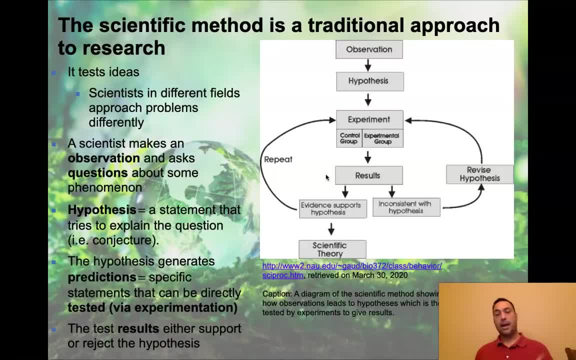 volcano right. Maybe it's not created by a giant impact crater, Maybe a giant asteroid did not create the Grand Canyon. But when you look down at the bottom of the Grand Canyon, you see the beautiful Colorado River moving through it and you think to yourself: maybe the river is responsible for the creation of this. 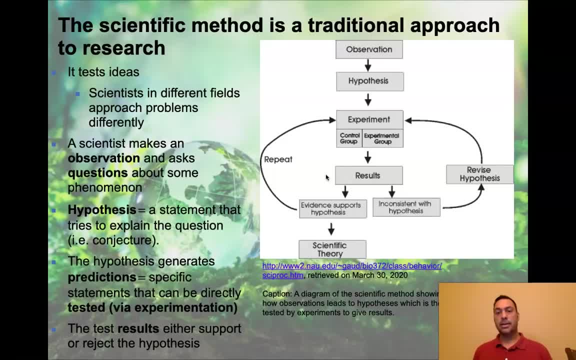 canyon And in fact science has told us that it is in fact the cause of the formation of the Grand Canyon. So we could then test those predictions, And the test results either support or reject the hypothesis. So, observation to hypothesis, right, The hypothesis is your conjecture, Then you do. 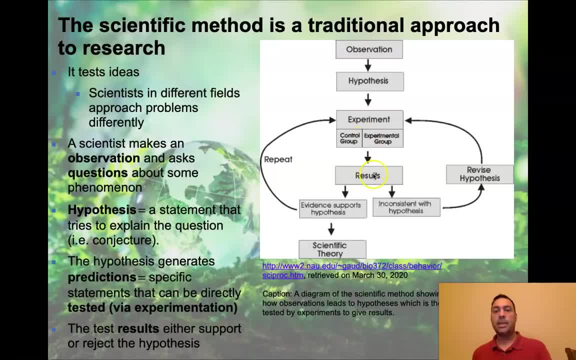 some experiments or you do some tests and you get the results. If it's consistent or supports your hypothesis, you repeat it. And if you keep getting the same thing over and, over and over again, that yeah, no, it fits, it fits every. 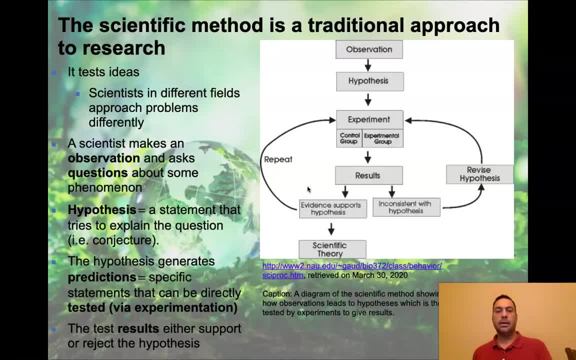 single time you do another test or another experiment. eventually, that could become your scientific theory, which will then become the accepted view of that phenomenon. right? People don't accept that the Grand Canyon is created by a giant volcano. They accept that it is created by the Colorado River. All of our. 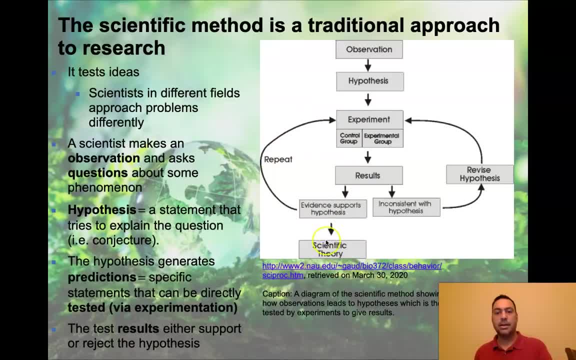 evidence supports that hypothesis. So that's our scientific theory. But if we came in here and we looked and we said we can't find the lava flows, but there's a tremendous amount of sand that's being deposited in the Gulf of California that seems to be from the Colorado River. 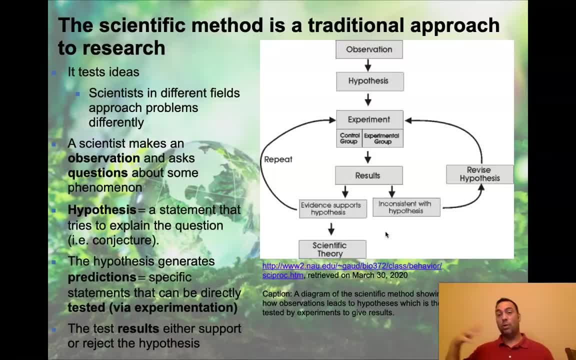 and the amount of that deposition seems to match roughly the volume of material that's removed from the Grand Canyon. maybe we need to revise this hypothesis. We do our experiment. We wind up in the right place. The goal is that, given enough experiments and enough time, we will eventually wind up with some. 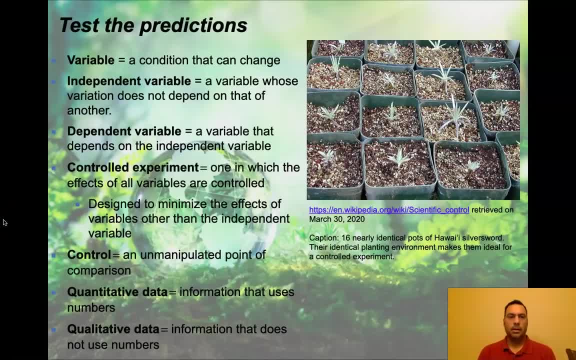 theory of that phenomena. All right. So when we're carrying out science, we actually need to be aware of some of them, some important parameters and vocabulary, so that we are able to keep track of everything that's going on. And so we're going to take a little bit. 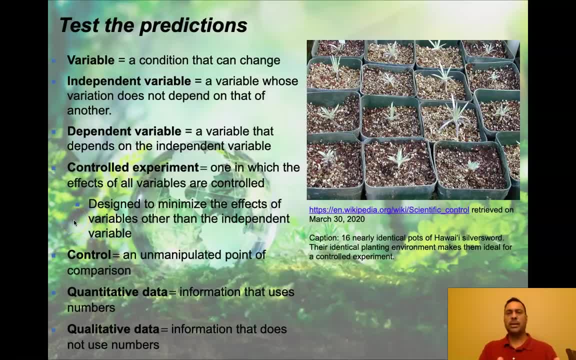 of time, because this is this is something that's going to happen a lot during the upcoming lectures. I'm going to bring these concepts up, so it's best to get them in right away. So the first concept is something called a variable. It's a condition that can change, It's anything that can change Now an 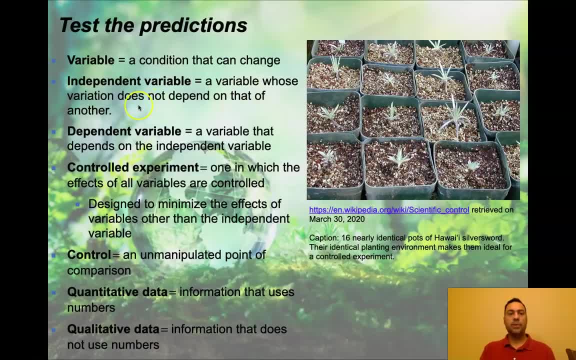 independent variable is a type of variable. It's a variable whose variation does not depend on that of another. In other words, it just simply is. It simply is independent, It doesn't change, It is not dependent upon something else, Whereas a dependent variable is a variable that depends on the independent. 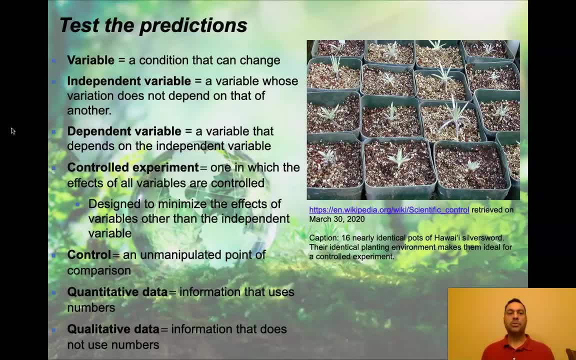 variable. So, for example, maybe the amount of water that is given to a plant, It might be an independent variable. It's a variation that does not depend upon another. It just simply is that value. So, for example, here we have a bunch of. 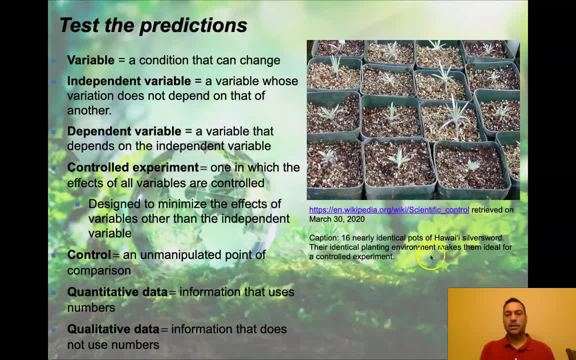 plants that are in a lot of little pots here. These are what they call Hawaii silver swords. They have identical planting and it makes them ideal for a controlled experiment, So we can do everything exactly the same. That gives us a good independent variable. Now the dependent variable is something that's going to be dependent. 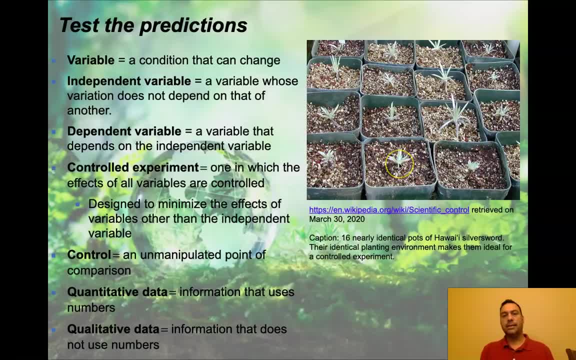 upon the independent variable. So, for example, maybe this particular plant has a slight difference in genetic structure or in genetics, So it might have a different outcome, But you water them all exactly the same, Right? so a controlled experiment is one in which the effects of all variables 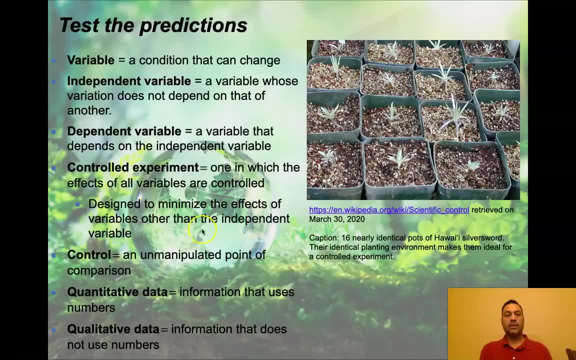 are closely controlled. It's designed to minimize the effects of variables other than the independent variable. In other words, if you want to see an effect, you want to make sure everything is exactly the same to the best of your ability, so you can measure an actual response to what you're doing. So a control is an 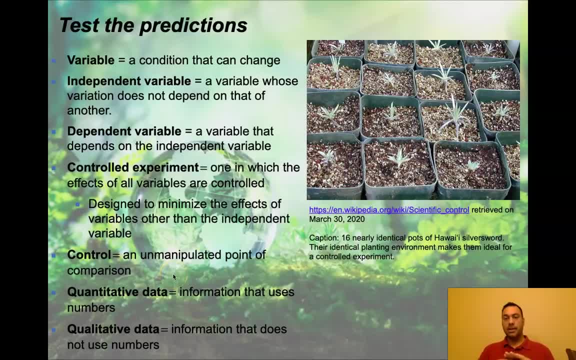 un-manipulated point of comparison. So as long is everything is the same and you do everything the same, the only thing you're changing is the one thing. the control shows you what the outcome would have been had you not made that change. There's two ways that this is. 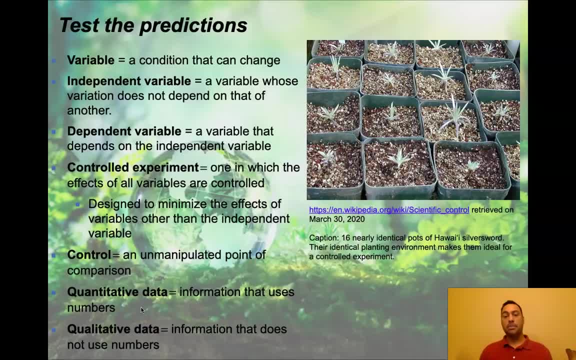 usually reported. You have quantitative data. This is something that uses numbers. right, You get an actual numerical output. For example, maybe you're measuring the height of plants, Or qualitative data that does not use numbers. Maybe it's a color, for example. Even in color, you can even use certain numbers by looking at. 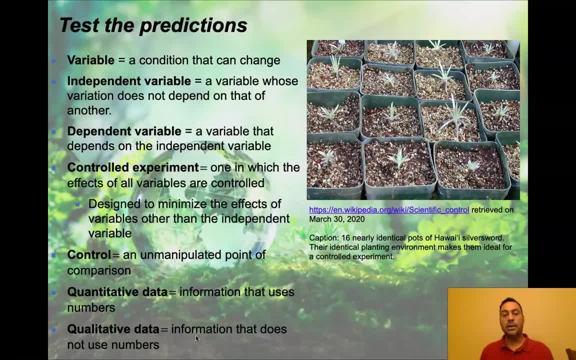 wavelengths and things like this. But you know, qualitative is another way of doing it. A lot of chefs that are doing cooking, they do a lot of qualitative data. Quantitative data when you're doing cooking school, for example, is a. 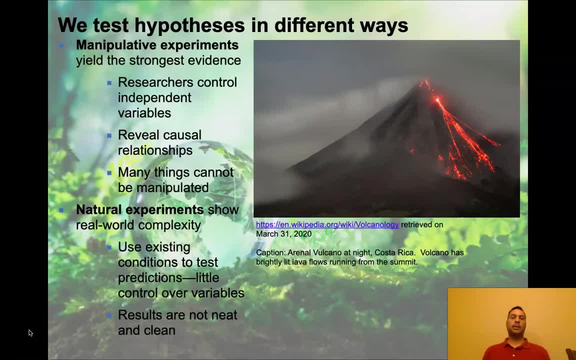 little bit more challenging, Alright, So we tend to test hypotheses in different ways. We kind of hit on this a little bit earlier, But you can do a manipulation. This is where you control the independent variables, And when you control the independent variables, you can reveal the 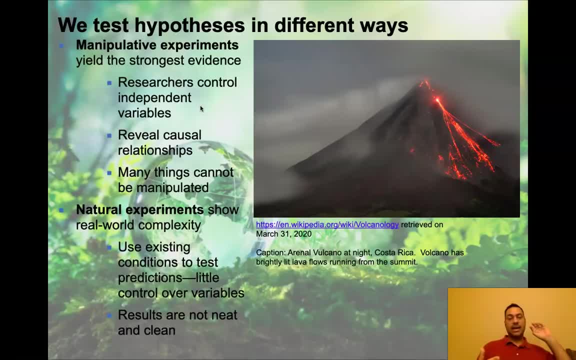 causal relationships. If I, if I, you know, if I hit a I don't know, hit a watermelon with a bullet, the watermelon is gonna break. But if I hit a watermelon with a, with a, you know, a sponge, it's not That kind of thing, And so I 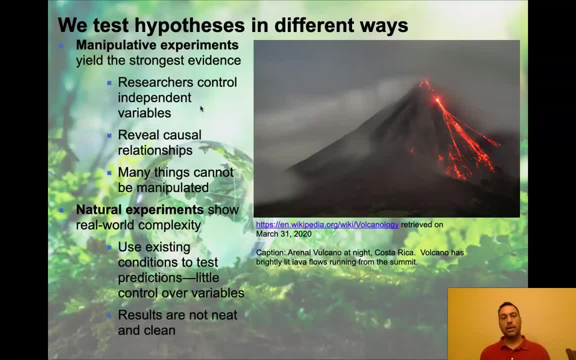 can actually put together these very simple causal relationships In medicine. this is, of course, a very big deal. Many things, however, cannot be manipulated, So that's when we usually do natural experiments. A classic example, something that cannot be manipulated easily, sometimes not at all, is something like a: 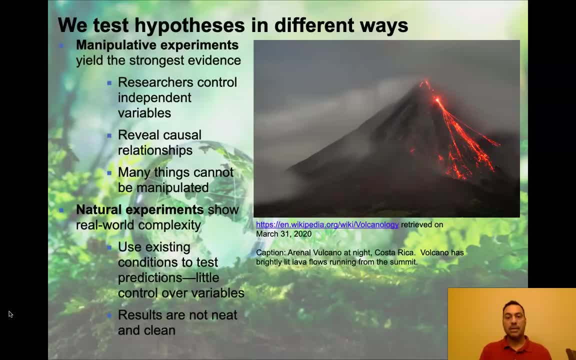 volcano. This is a volcano in Costa Rica. at nighttime, You can see the lava flows flowing down from the summit. You wouldn't want to get near this thing. It would probably kill you if you tried. So in this case you use existing conditions. 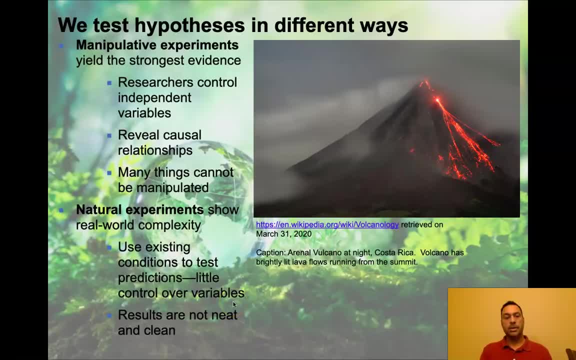 to test the predictions, Little control over the variables and the results are not neat and clean. You know, sometimes you'll you'll look at something like a volcano, like this, and you can't get exactly the data you want. but you can get a kind of an estimate. 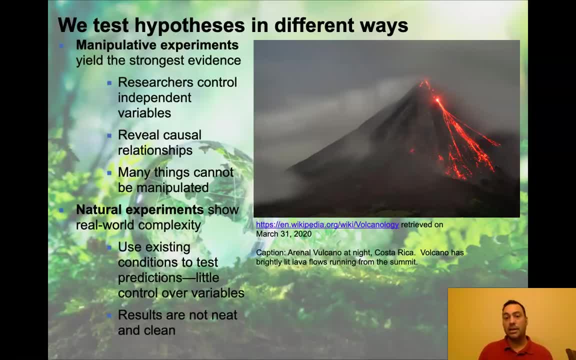 on what it might be doing. Maybe it's the type of lava that's coming out, the kinds of gases that are coming out, the temperatures. There's ways to get good measurements on these things, but there's always sometimes some information that's. 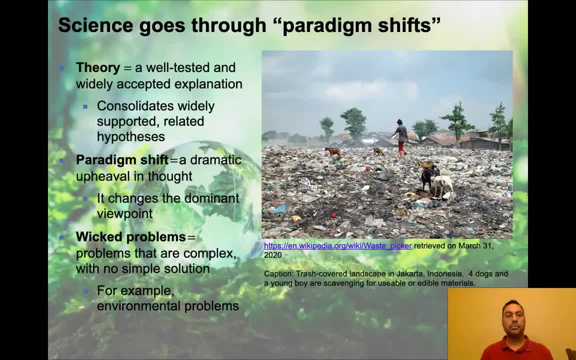 not as clean as we want it to be, So science tends to go through these things called paradigm shifts. These are large changes that happen, And so we start off these theories. We talked about these earlier, right, So it's a well-tested and 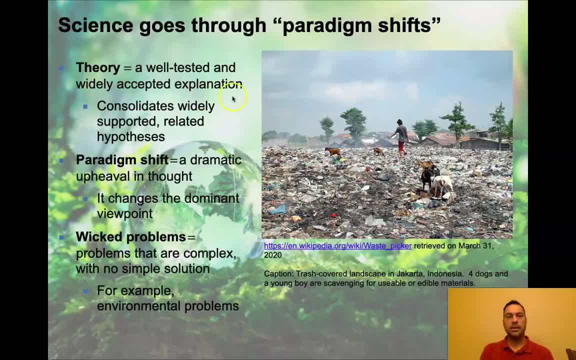 widely accepted explanation of something of a phenomenon that's happening And it consolidates widely supported related hypotheses. In other words, it's something that brings everything together and it makes everything understandable until something you know undermines, that completely changes it. When that changes, that's called a paradigm shift. It's a. 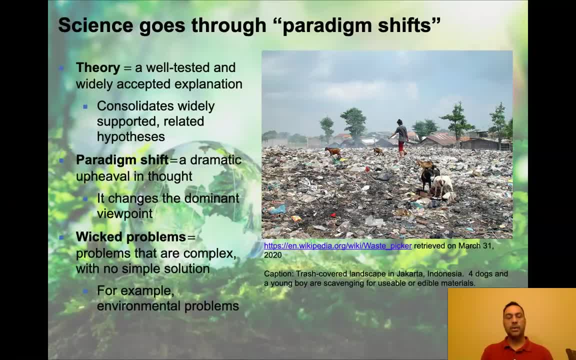 dramatic upheaval in thought that changes the dominant viewpoint. The classic example of the paradigm shift happened in geology, for example, where they discovered that continents on the planet Earth, on the planet Mars on the planet, the Earth on the planet Mars, on the planet Earth, on the planet Mars on the planet. 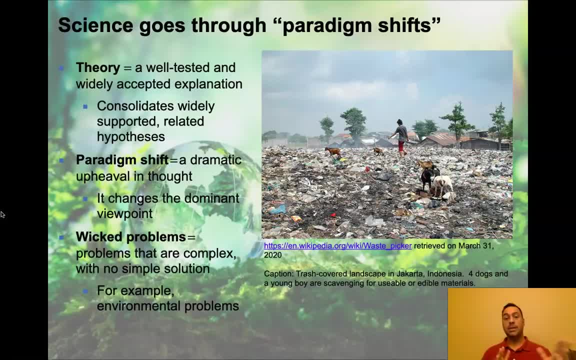 Earth actually move around as well, as ocean basins tend to evolve over very long periods of time. Prior to that, there was no concept of this. It didn't seem like the continents could move around on the surface of the Earth And everything. 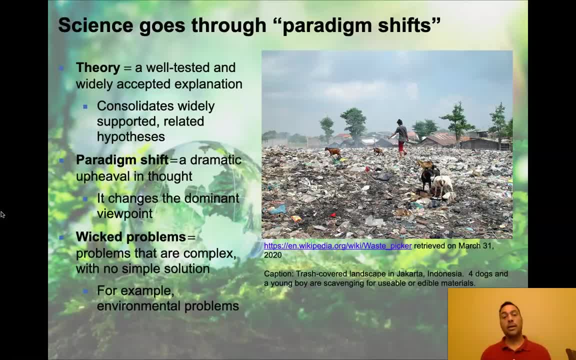 was explained using a completely different system. We now know that that old system isn't accurate. It was done away with. It was replaced by the current plate tectonic system. Similar things have happened in biology: the understanding that genetic information is transferred through DNA and RNA as a 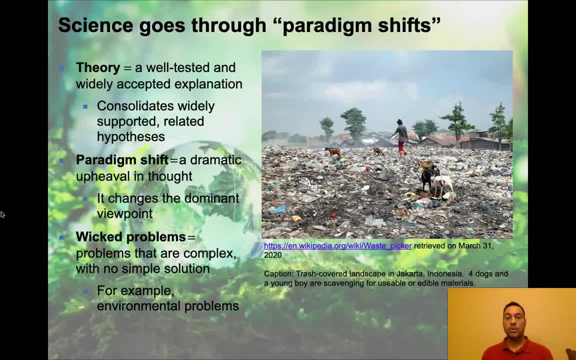 opposed to other means, was a huge eye-opener for many people studying the biological sciences. Now, some problems are what we call wicked problems. These are extremely complex problems that don't have any simple solution. In fact, there might not even appear to be a single solution to any of it, And 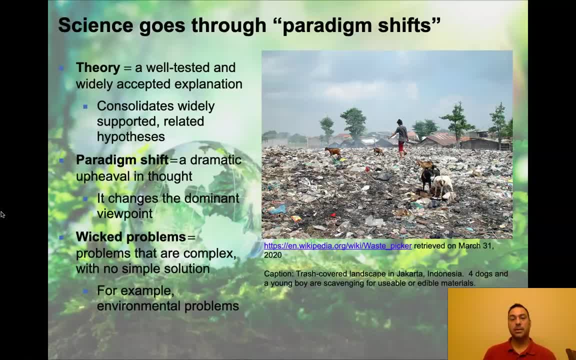 environmental problems are classic examples of wicked problems. You know, here we see this is a trash-covered landscape in Jakarta, Indonesia. The boys out here scavenging for usable and edible materials. The dogs are out here eating whatever they can find And, in a weird way, them being out there. 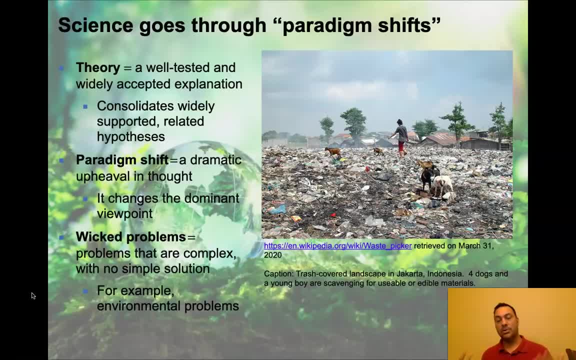 doing this helps clean the landscape, But in another way, it also encourages more poverty, and this is obviously not the way you want to live, right? So wicked problems happen, whether they be economic problems, political problems, And in case of an environmental problem, who's responsible for this cleanup? right, How? 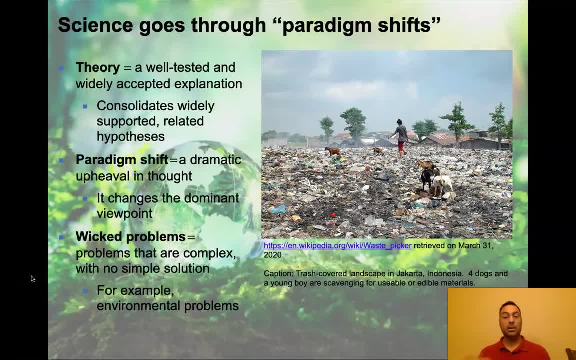 did the trash get here in the first place? Is this a public policy problem? Is it a cultural problem? Is it a political problem? Is it a cultural problem? Is it an economic problem? Is this a political problem? Is it a cultural problem? Is it a? 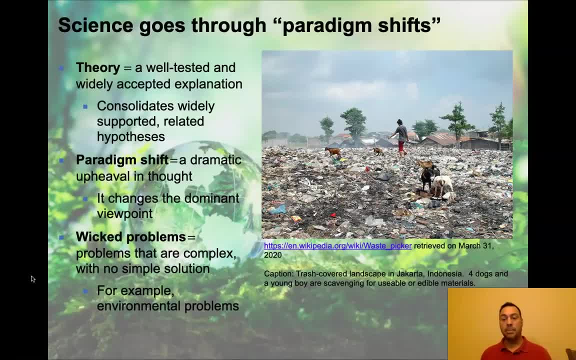 problem? I don't know right. It depends upon how we go about solving or looking and analyzing these, these issues. In fact, for these dogs it's not a problem at all, right, Because they actually have a free meal. All right, so let's start. 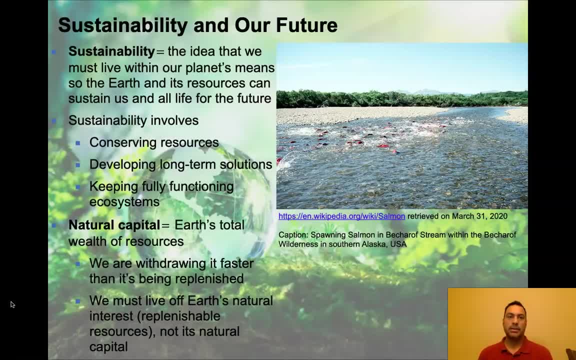 introducing another word that you hear a lot when it comes to environmental science. It's called sustainability. Sustainability is a concept that a lot of people misunderstand. They usually think that it meanssustainable means conservation. It can mean conservation. It's one of the things that we 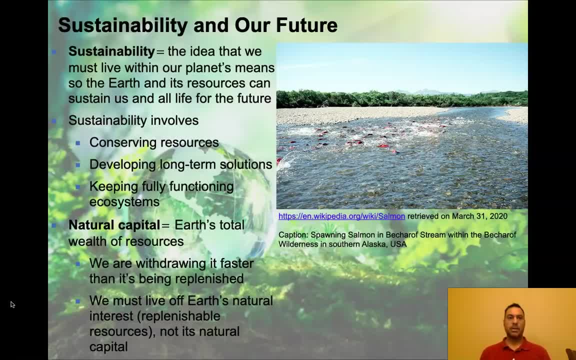 frequently see, but it's not the only thing that we see when we talk about sustainability. So sustainability is the idea that we must live within our planet's means so the earth and its resources can sustain us in all life for the future. So basically it's: what can we do to make sure that the ecosystems 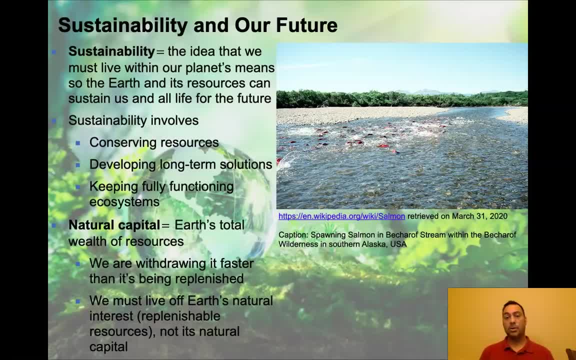 continue to provide what we need so that we can continue on the path that we currently are on. If we don't change things, obviously if we're at 1.7 percent, we're not going to be able to do that. If we don't change things, obviously if we're at 1.7 percent we're not going to be able to do that. If we don't. 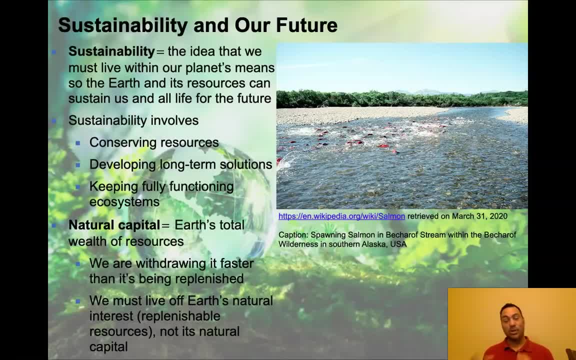 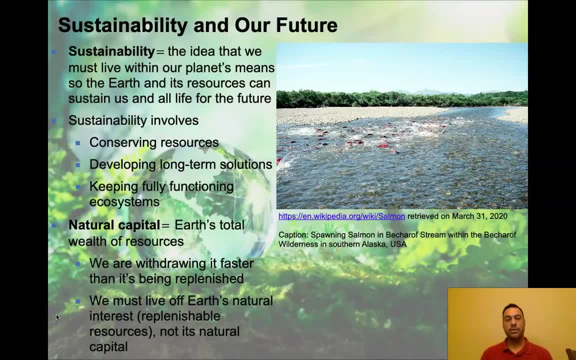 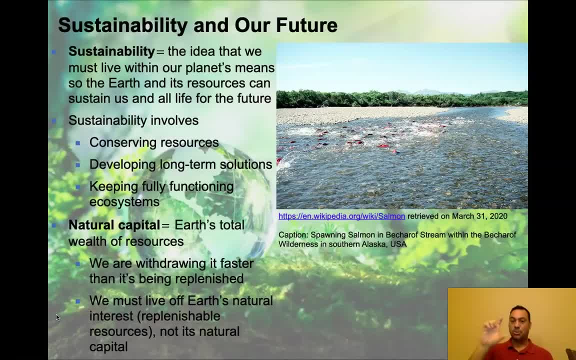 every single month, You're also spending the, the actual principal that you put in. Eventually, once you draw down the principal, you don't have either. You don't have, you don't have the interest income and you don't have the principal. That's the same concept here of natural interest. It's Earth's replenishable. 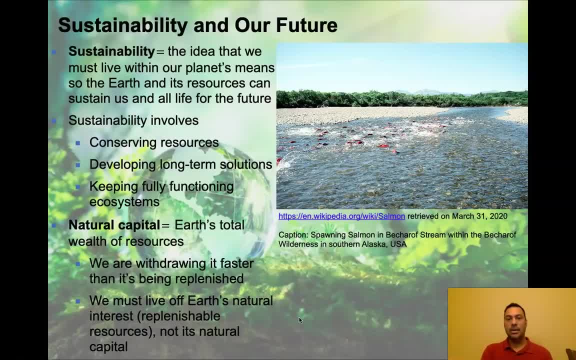 resources, Something you get every single time without having to do anything. Classic example of this natural interest that they're talking about are: these are salmon in the wilderness of southern Alaska. They come back every single year and you can harvest approximately 50% of them every single year sustainably. 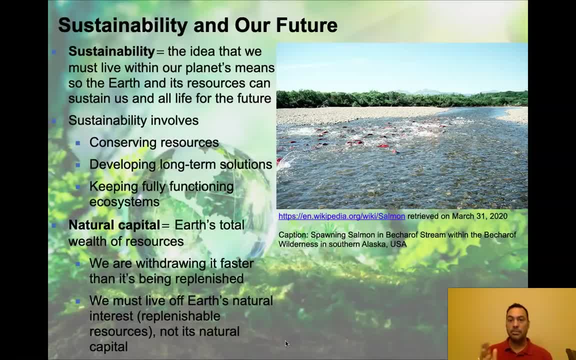 forever. But if you take more than that, you will impact this. And, of course, if you impact the rivers, maybe you take the water away or you put a mine in the area and the mine pollutes that river. then you lose the salmon that way as well. So 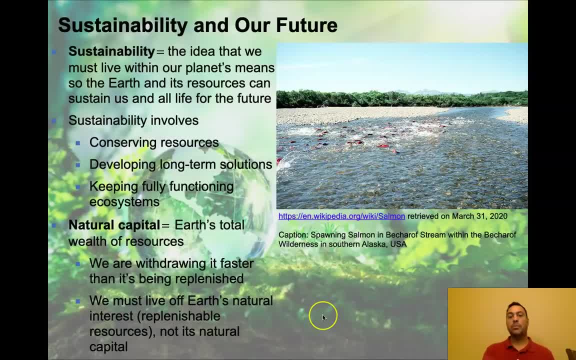 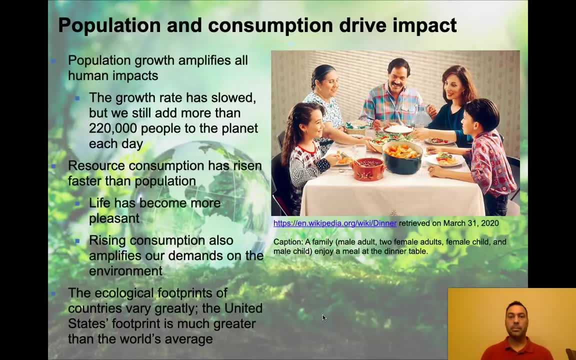 this is the natural interest that they're talking about: The fact that we could draw on that salmon every single year as a resource without diminishing it, as long as we're careful. Now, a population that's in the wilderness of southern Alaska population consumption definitely drive the impact As we get larger we have. 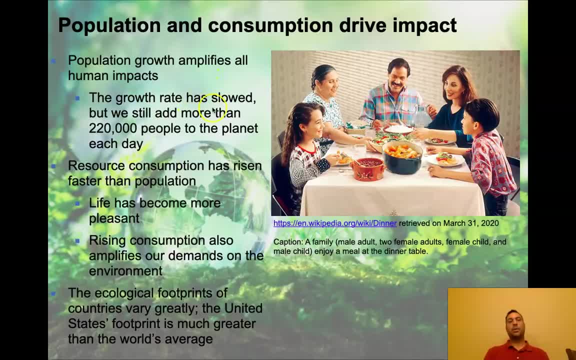 larger impact. So population growth amplifies all human impacts. The growth rate has slowed, but we still add more than 20 or 22 or 220 thousand people. Wow, I understated it in my mistake: Two hundred twenty thousand people to the. 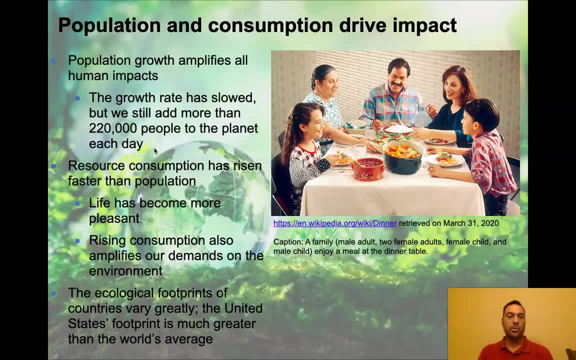 planet each day. That's a number I looked up right before recording this lecture. So resource consumption has risen faster than population. because people are becoming more affluent, right, Life has become more pleasant. So as those people come online and join the rest of us in the economy, they're 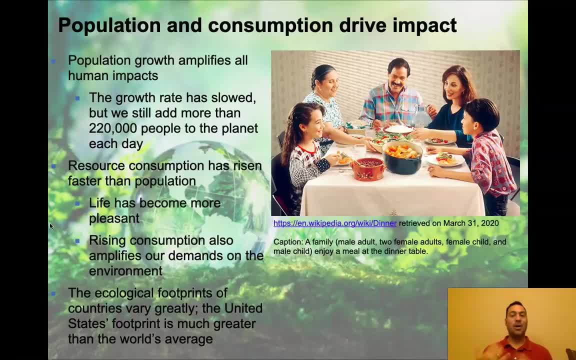 also wanting to live better lifestyles. They want air conditioning, They want farms, They want to have a nice school, They want good libraries. and this isn't just in the United States, This isn't just in North America. This is worldwide. This is happening and eventually they're going to want these things everywhere. 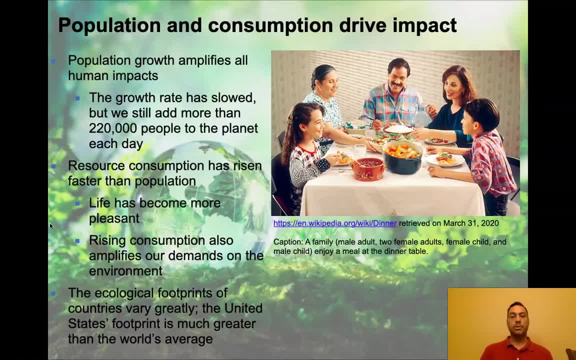 and get those things everywhere, but that requires resources. So rising consumption also amplifies our demands on the environment, which is one of the reasons why we're seeing so much environmental degradation happening at exactly the same time. So here we see kind of this classic family over here. but think about 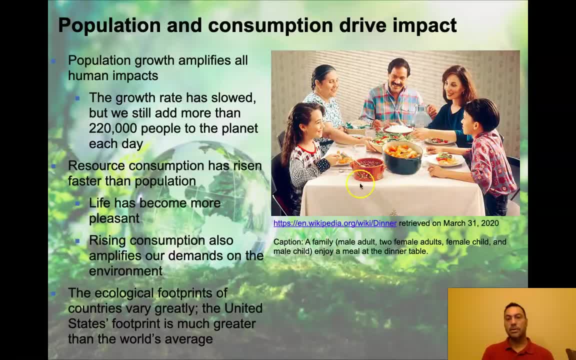 the amount of resources it takes to clothe them, to put this tablecloth on here, to make the pottery, to produce the food that goes into just a single meal. right, just to make that image exist with all of its attributes, And you can see. 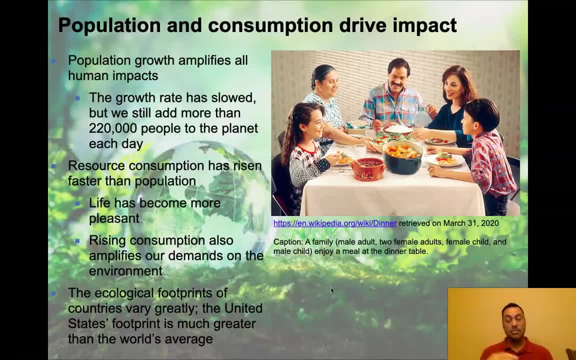 they're all happy and they're taking a great family photo together, but the issue is still the same: It requires a tremendous amount of resources for the earth to be able to produce just that single event to have it happen. So the ecological footprints of countries vary greatly. as we talked earlier, the United 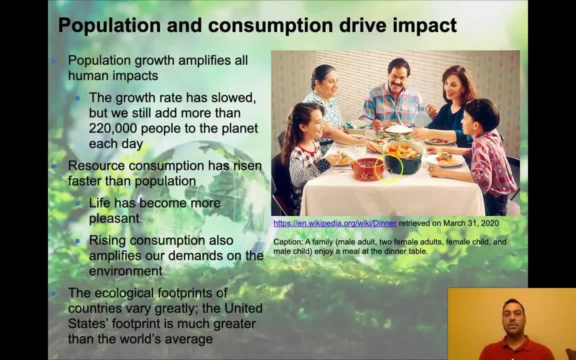 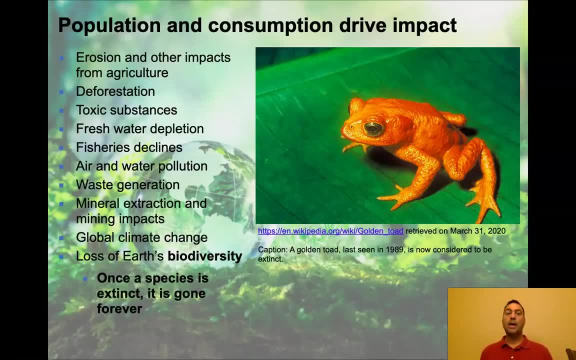 States footprint is much greater than the world's average. This is a typical American family today as we know it. So what are some of these impacts? What causes some of these impacts? Well, erosion and other impacts from agriculture, the dry impact, deforestation. 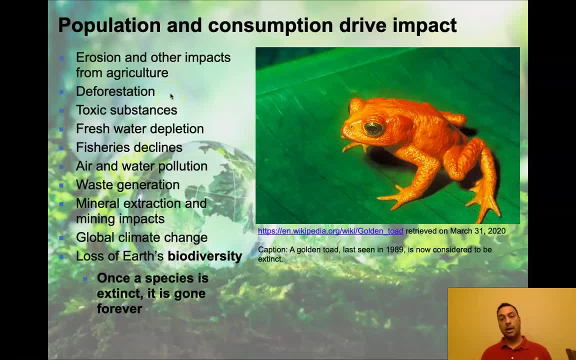 our disaster and glitches. So what causes that? Well, we don't need just any kind of desire to cut down trees, not only just for the lumber, but also because we want the space. Trees tend to grow in very favorable areas, especially in flatlands. Toxic substances are. 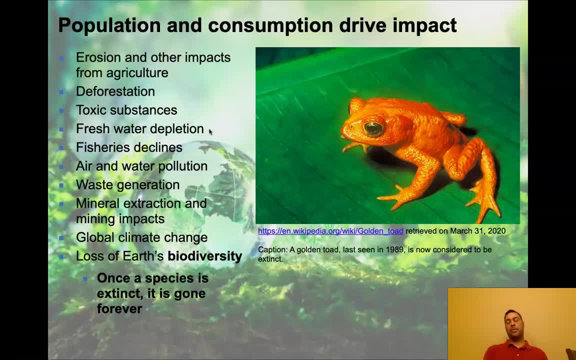 becoming a major issue- Freshwater depletion. In fact, I say it all the time and I'll say it many times during this class: freshwater is worth much more than gold, So the desire to go and get access to freshwater is huge. Fisheries declines, air and water pollution, waste pollution, mineral. 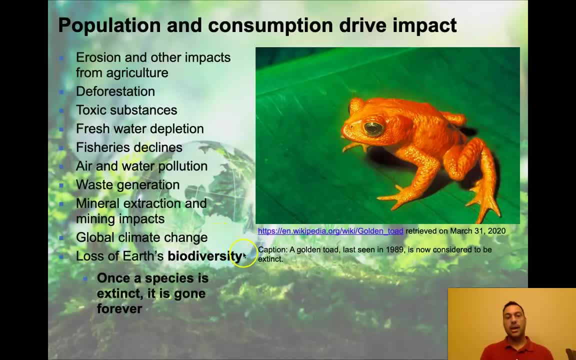 extraction and mining impacts global climate change and, of course, loss of Earth's biodiversity, And we're going to talk about that a lot. That's a really, really big deal. Now, once a species is gone, it is gone, or gone extinct, it is gone forever. So biodiversity is a big deal And you. 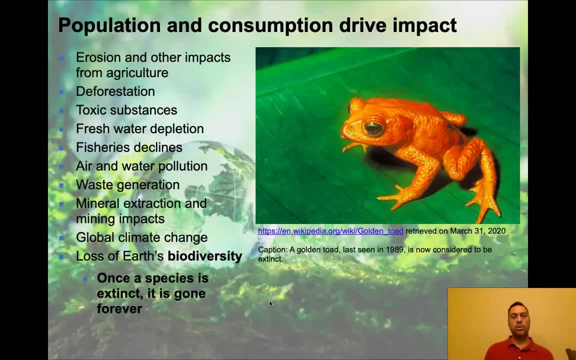 might not think of it as a big deal. Like you know, for example, who cares if a toad goes extinct? Aren't there other toads? Well, maybe not the kind of toads that we need them to be All right. 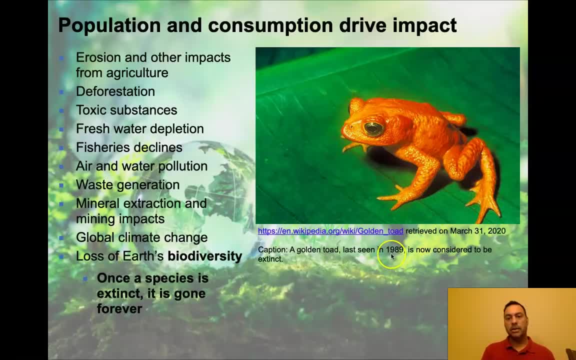 So we're going to talk about that a lot, And we're going to talk about that a lot, And we're going to. So this is the golden toad. This is an animal that's been completely absent from human eyes since 1989. It's considered to be extinct. So this is a picture from before 1989. 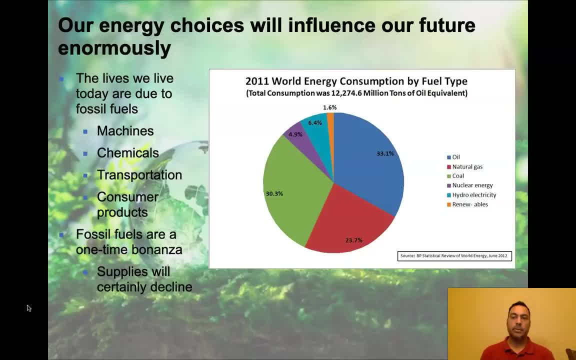 In terms of things that we do on a day-by-day basis, it's usually our energy choices that tend to have the largest single influence on a day-by-day basis. So the lives we live today are due to fossil fuels, Everything, all the conveniences that we have, the machines that we have. In fact, in order, 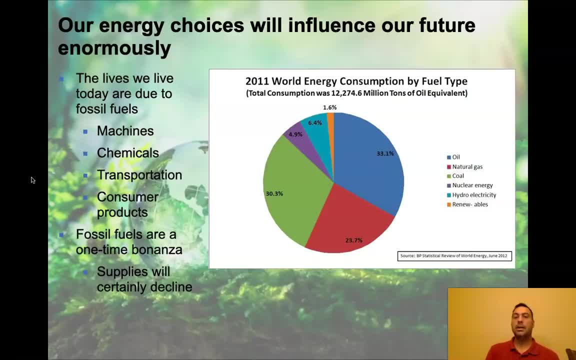 to produce steel you need to take fossil fuels, not only to heat the iron, but you actually take part of the fossil fuels and you use it to alloy itself with the iron to make steel Chemicals. a lot of the fertilizers that you guys use on your plants actually come from petroleum. 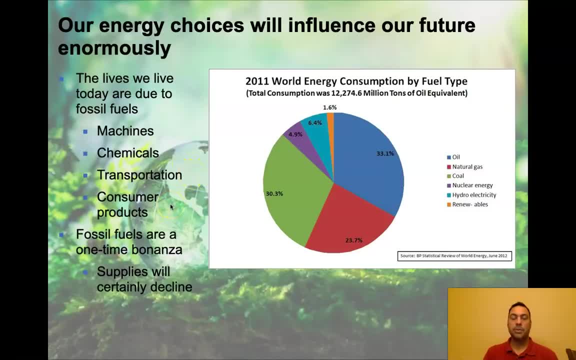 Transportation, of course, comes from petroleum Consumer products. a lot of the makeups that people like to wear on their face, a lot of the clothing that they like to wear, also come from non-renewable resources and things like petroleum And fossil fuels, of course.